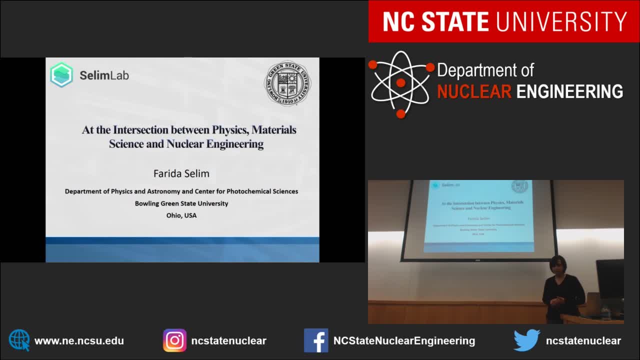 Then she worked as a postdoc researcher at Idaho Accelerator Center, Then as a research assistant in a professor in Washington State University, And she is currently an associate professor at Bowling Green State University. Professor Selim has published more than a hundred peer-reviewed journal articles. 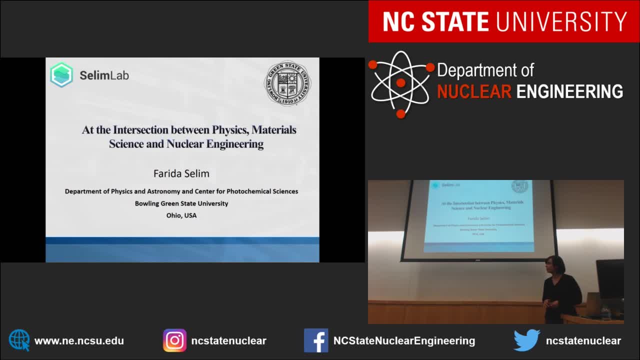 She has three patents. She is known for inventing the new positron annihilation spectroscopy technique, which is called the gamma-induced positron spectroscopy. I believe you are going to mention a little bit about it. Yes, probably one slide. 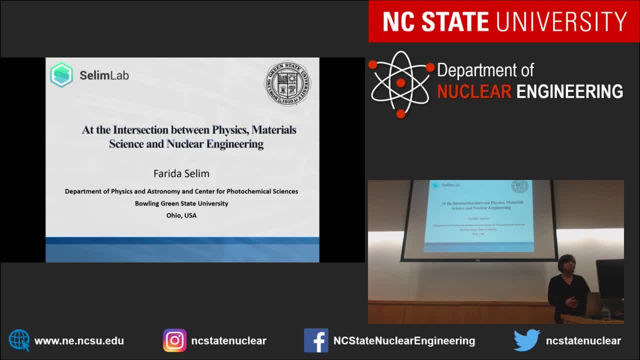 Which has been adopted and used for developing new positron facilities in Dresden, Germany, in Japan and in India. She has expanded positron applications to new areas in material science And currently she has active research programs on electronic photonic materials with a focus on growth and characterization of semiconductors in wide bandgap oxide. 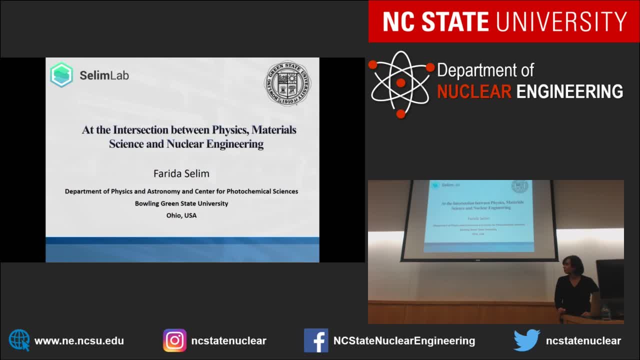 But I will add to that the structural alloys now, Because Professor Selim is actually a collaborator of ours on a new project where we look at radiation damage and corrosion in structural alloys for general reactors. So she currently serves as an advisor on three international committees. 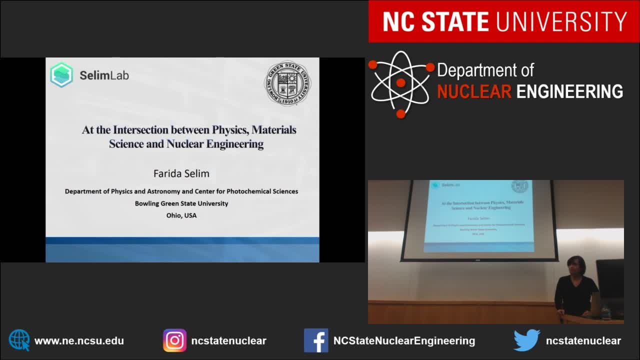 The International Advisory Committee of Positron and Positronium Chemistry, The International Advisory Board on Positron Studies And the Advisory Committee of the International Conference on Positron Annihilation. So please, let's welcome Professor Selim. Thank you very much. 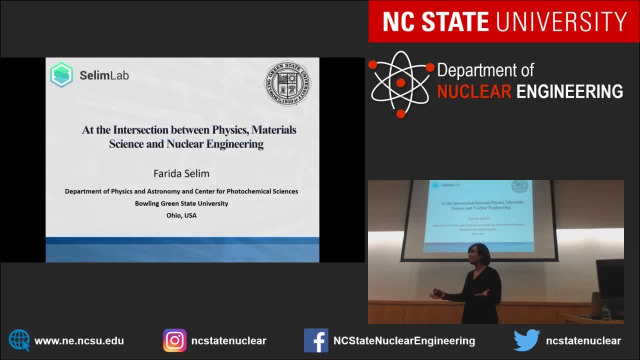 Thank you very much for the invitation and for the nice time here. It was really very nice to visit this campus here. I visited this campus a long time ago And I'm really glad to see the campus here and everybody. So thank you very much again for hosting me here. 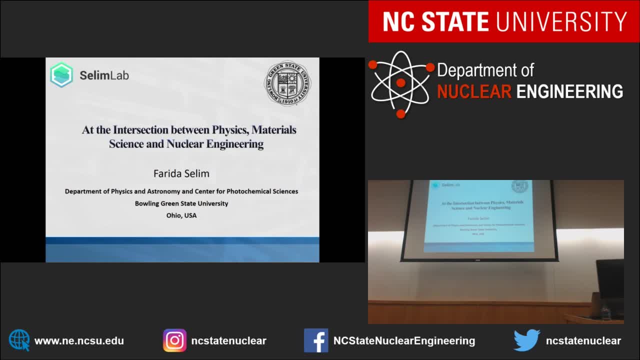 And hopefully I don't disappoint you. My background again is physics, So I'll try to get some stuff which is related to nuclear engineering, But most of my work I'll probably give you a little bit idea about what we do in our lab. 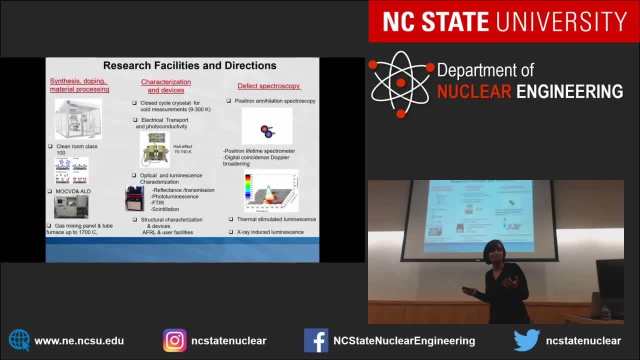 So you know I'm not really a nuclear engineer person. But then I'll tell you where is the intersection Between, like I said, physics and material science and the nuclear engineering. So in our lab very much we're doing, We grow fundamental study and applied research in what we call wide band gap oxide. 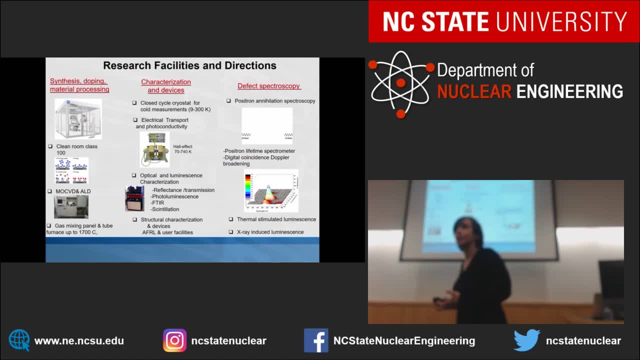 But we have also, like Jamal mentioned, We have some interesting structural material and engineering material. So we do sensors as material, We grow nanostructure. We have clean room plus 100 in our lab. We have metal, organic chemical vapor deposition. We can do a bit axial growth of oxide for semiconductor device and for photonic application. 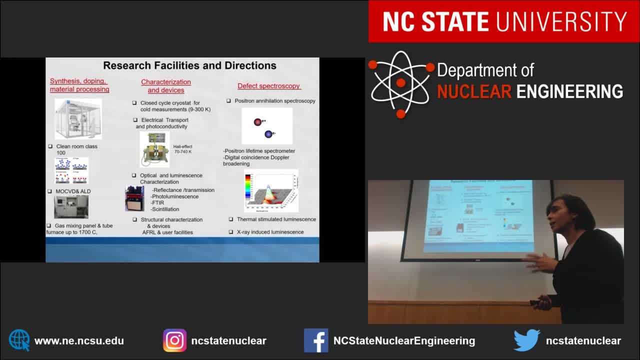 And we do a lot of characterization, from electrical transport measurement to luminescence and optical characterization. And important field of ours of course is defective spectroscopy, And for defective spectroscopy we use positron annihilation spectroscopy as a main technique And thermal stimulated luminescence and other optical technique. 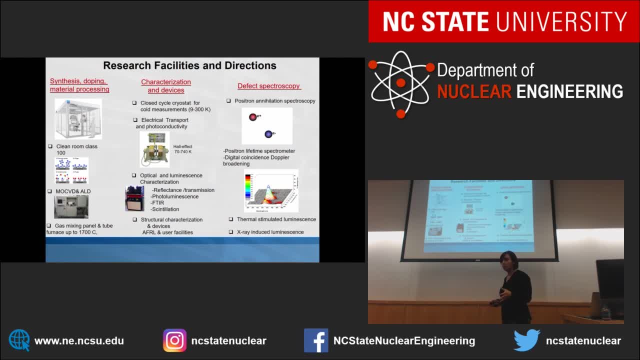 Positron. probably my focus is going to be here on positron, Because I don't know if you guys know you have a nice positron facility here. I don't know if people are aware of this or not. And then positron has a lot of application. 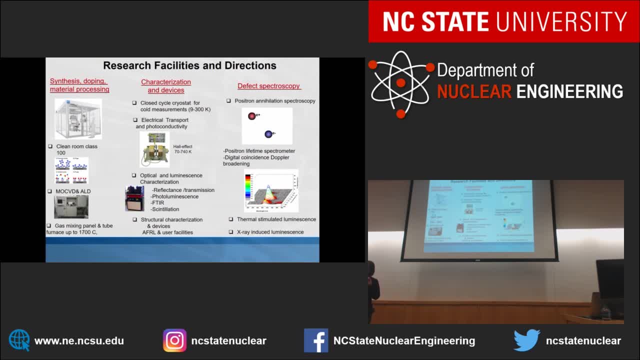 And it has been always one of the interesting technique to look to nuclear material and to study defective material. So it is really, if you look to the literature, Positron has been really useful to look to this kind of study. So my focus is going to be on this part. 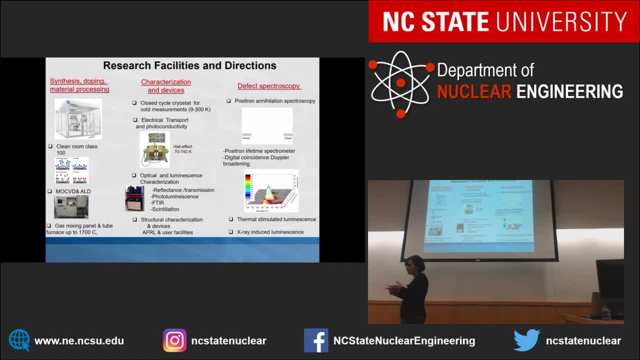 To introduce to you what's positron annihilation as a physicist, What is positron, How positron is used to study defects. And then I'll talk a little bit about something else I do which is new to detectors: Nuclear detection stuff. 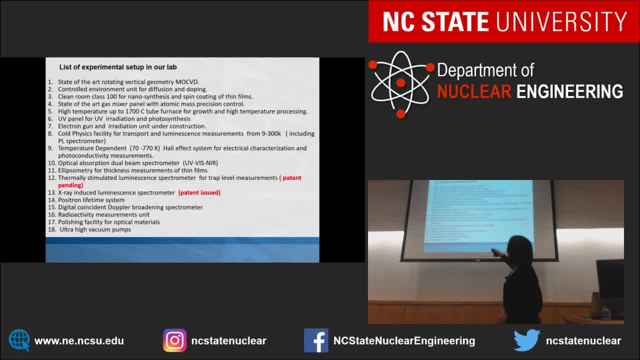 So this is very much is most important. But this is some of the list of examples. This is an experiment set up in our lab. When I go to colloquium, I always show people because they are interested in our facility. So this is some of the stuff we have in our lab. 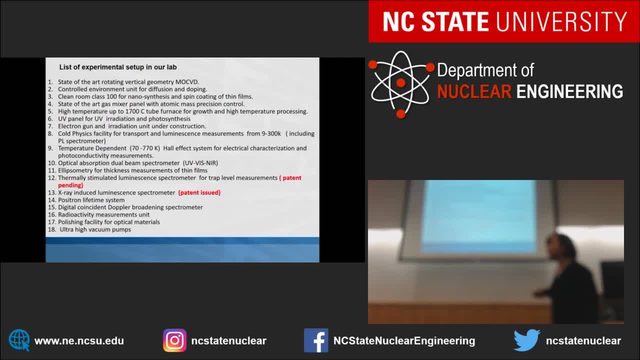 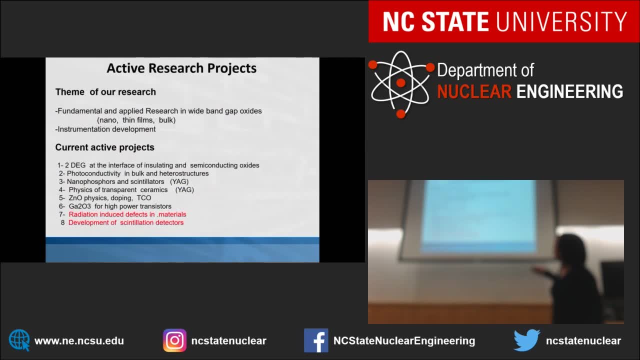 But you probably see most of them. it's really electronic and photonic stuff, But we have defect spectroscopy, A big part of this. So this is some of our active research project And my focus, as I said, is going to be radiation induced. 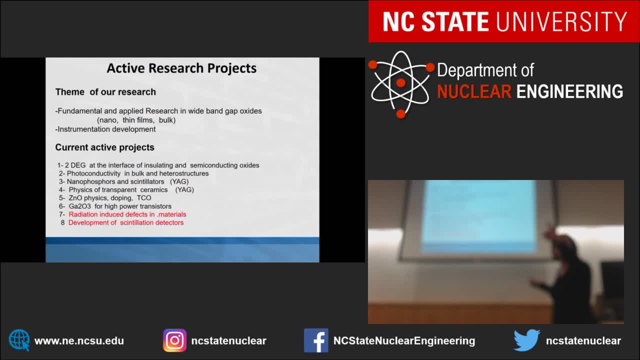 So radiation induced defect in materials. This is my cooperation with Jamal here. This is what we do with it. We do positron spectroscopy, We do TM And this is where it's called our cooperation. So I'll talk a little bit about that. 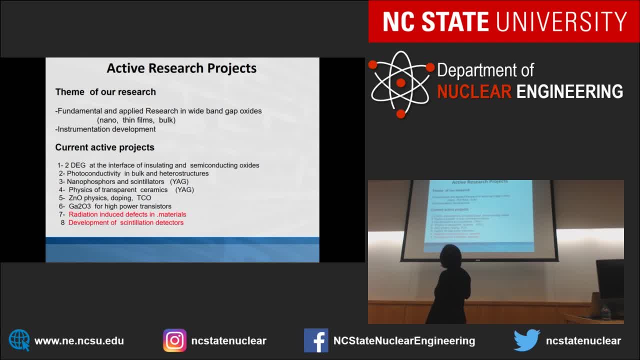 This is why I'm going to talk about study of defect here, And the other part is development of centralization detector, And I think you have some area of here too, And I'm going to mention at the end about neutron transmutation And dobing. 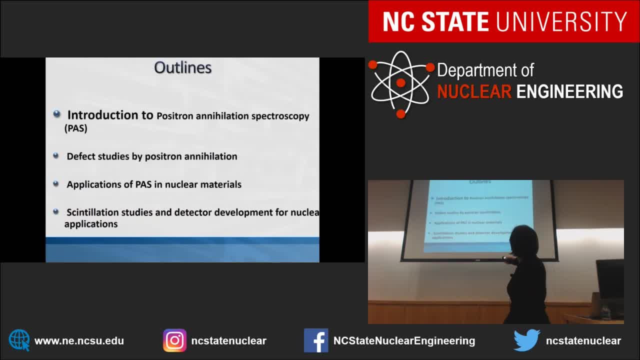 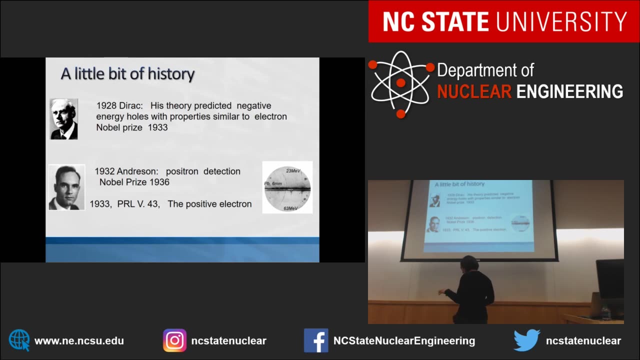 So let me start. I already told you the outline of my talk before I show it. So introduction to positron annihilation, Defect study And application of. So yeah, Let me give you a little bit of history about. So I assume nobody put no positron here, right? 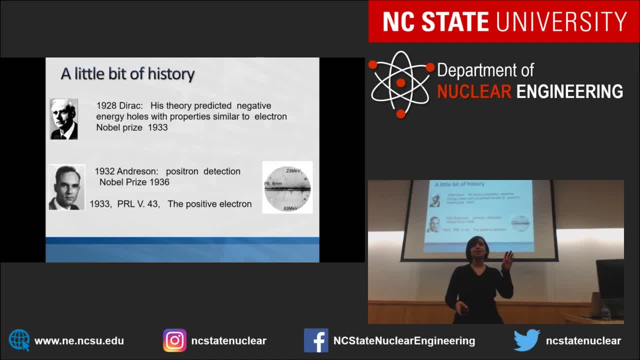 Except you, Yes, So positron is a positive electron. So you know electron, Everybody know electron. So possibly positron is a negative, Is a positive electron Where it starts. Let me start with a little bit of history. So if you know direct equation in quantum mechanics, 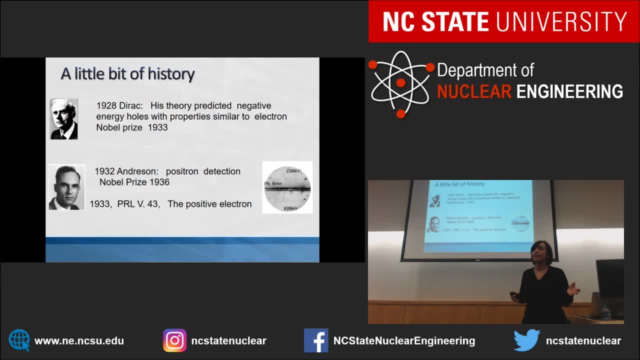 So direct equation He actually solved. with the equation He get negative energy solution. So he said this is like negative Positive electron. He found the hole with properties similar to the electron, So this was just his theory. And then Anderson, He measured actually the positron in 1932. 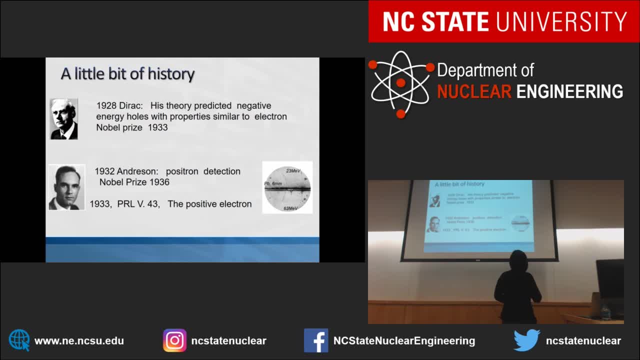 And this is the first. This is the first image actually For positron detection in a cloud chamber. So this is how it start. The positron And this guy get Nobel Prize. The two get Nobel Prize actually For the discovery of positron. 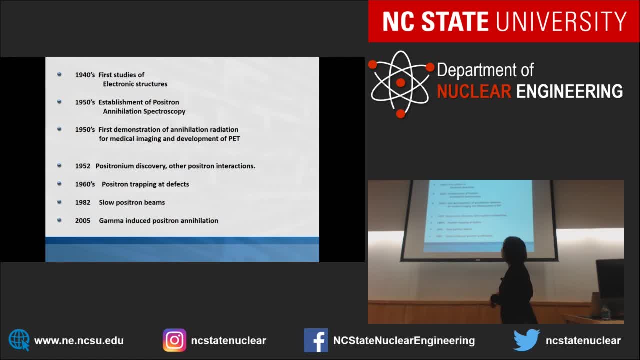 And after this, People shows that you can use positron To study electronic structure of material And I'll show you that it's been really One of the very important Method for this And then established to study Positron defect in 1950s. 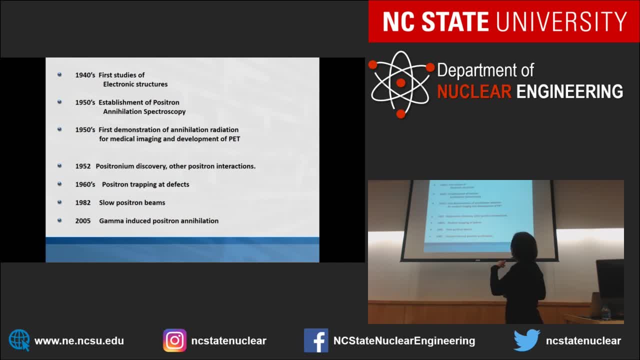 And then it go to Positron emission tomography, Also around this area in 1950.. So you're familiar with Positron emission tomography right In medicine, The positronium recovery. I'll tell you a little bit about it. 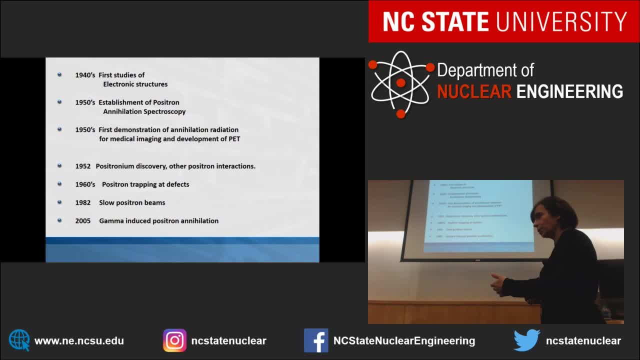 Positronium being too right too. You're developing positronium Right Facet. Then I'll talk about The different technique in positron, And this is very much how it's How it's going through the history. 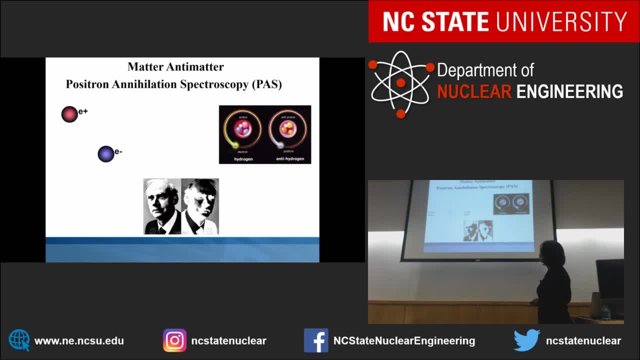 So Again, Positron annihilation, spectroscopy. The word positron annihilation, it mean It annihilate. So why? because it's antimatter, If you know any matter, and antimatter Proton, antiproton, positron. 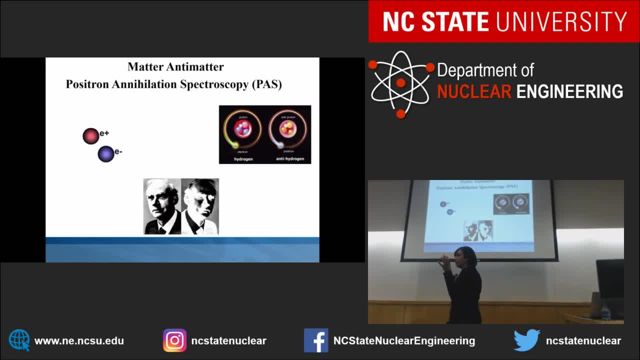 Electron when they meet, annihilate. They completely Disappear, The particle disappear And you get energy Positron again. Electron is the most elementary particle. So when we talk about positron electron annihilation, This is a very fundamental actually. 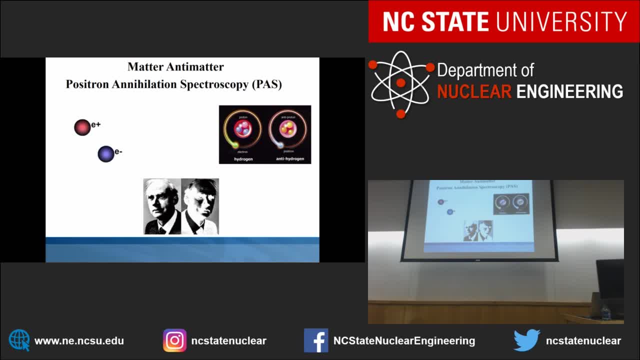 Matter, antimatter interaction. So for us the physicists, There's a lot of interesting physics there You can study when you study the interaction Between electron And positron Photon here, So the electron, positron As soon as they get close. 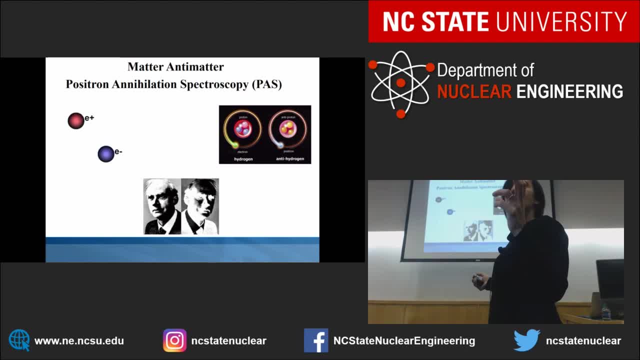 They completely disappear And you get two 511 photon. Are you familiar with this number 511?? 511 is the rest of mass energy Of the electron. This is 511 kilo electron volts, And then we get exactly 511. 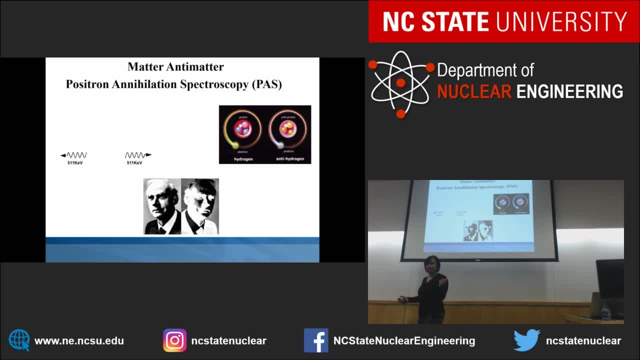 Two photon. What's interesting in this? This is: You're familiar with the Einstein equation. Right Then this positron electron, Positron electron annihilation Is actually very. It's the best, The best demonstration For Einstein equation. 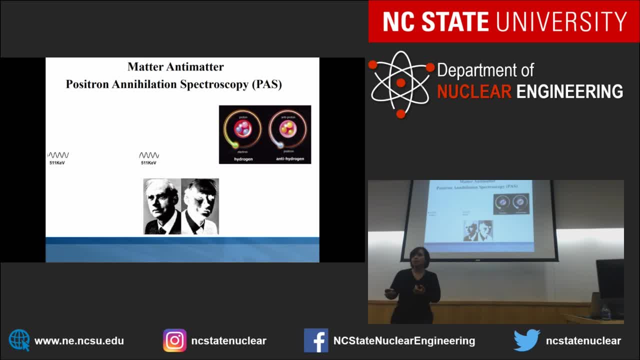 E equal m c square. Why? Because in nuclear reaction- You see part of the matter- Are transferred into energy Right And you get this amount, Huge amount of energy. And in electron, positron annihilation You convert 100% of the mass. 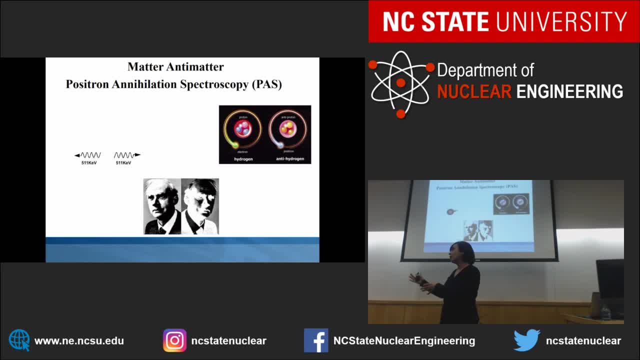 Into the energy, So all of the mass here And convert it to energy. So I always say This really shows the Between matter and the energy Are the same And we see the opposite process. We see also We can get from the two photo. 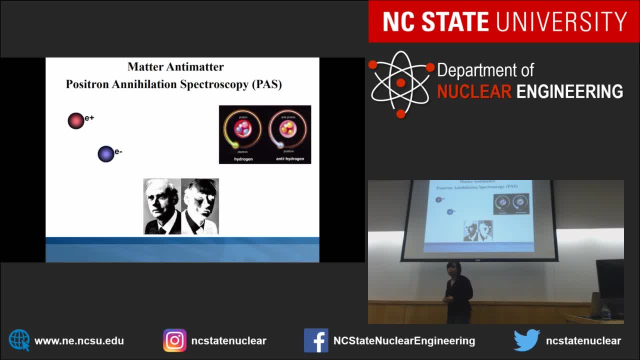 We can get electron and positron, What we call the pair production This way. What we have here, Hydrogen and antihydrogen- There is a large, There is a big work In certain lab To generate antimatter. 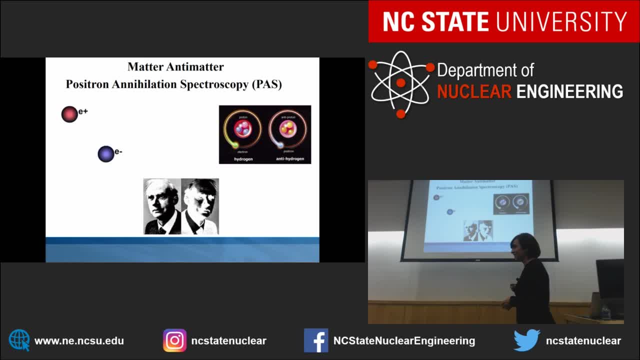 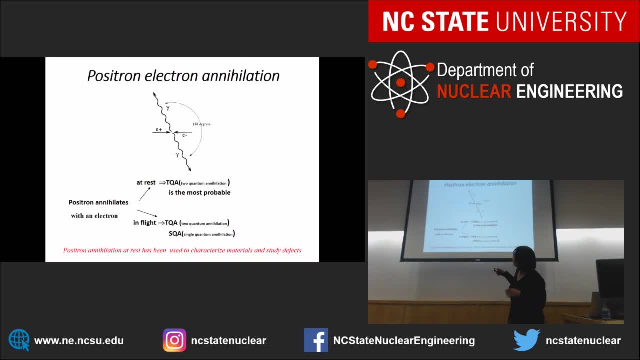 As a hydrogen and antihydrogen. There is a lot of This is. This is a joke, of course. Okay, So I don't want to talk. This is again the physics of When they annihilate Energy, and we call this. 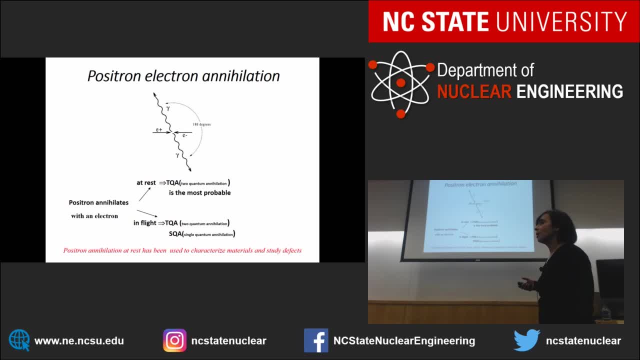 Positron annihilation in flight, Or they can annihilate When they have no energy, So zero kinetic energy. This time they give exactly two photon And each one has 511 kiloelectrovolts. So let me look to. 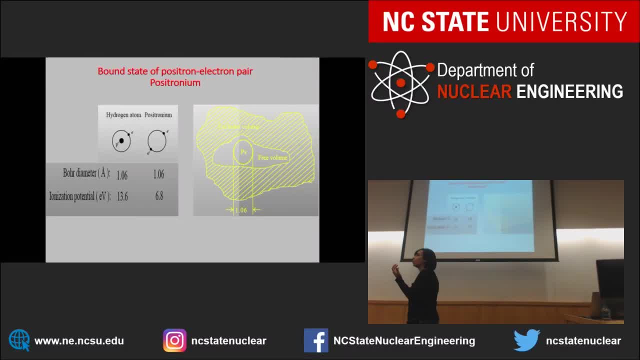 This also I have to mention to this. Have you heard about this before? The positronium. This is really the Sample type of matter in the universe. It's not the hydrogen atom, It's the positronium. So the positron is combination of 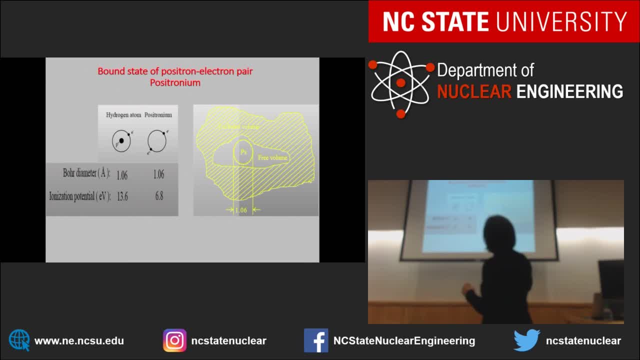 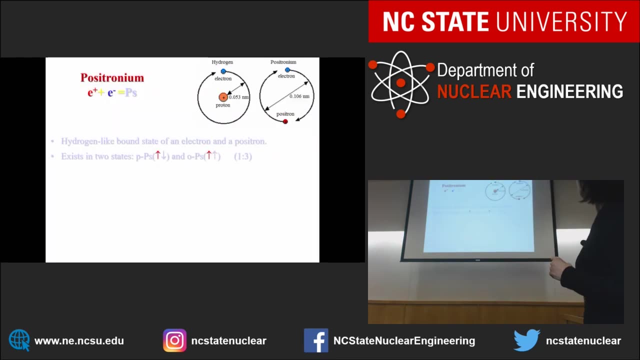 Electron and positron. So these are combined here, Similar to the. They have the radius, The same radius of hydrogen atom. So here is the electron positron And here is the hydrogen atom. If you look to their properties, I said They have the same Diameter. But positronium don't live too long Because it's the annihilate. It don't live. It depend of the spin state. Some in quantum mechanics We call the spin of the particle. The spin can spin up or spin down. 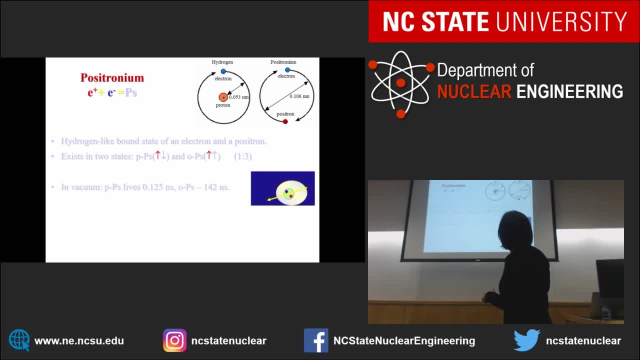 So if you have The electron positron here, If they have Similar, Similar spin, They form Also positronium. If they have Different spin up and down, They form And the bar of positronium Live 125 seconds. 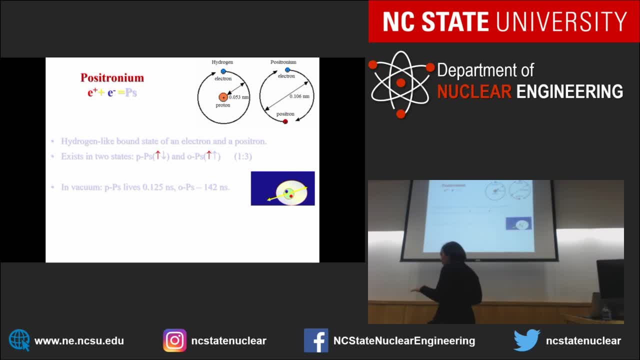 Also, positronium Live only 142 nanosecond In vacuum. The bar Live 125 picosecond. So this is very much We just want to tell People always about, Because this is really the simplest type Of atom. 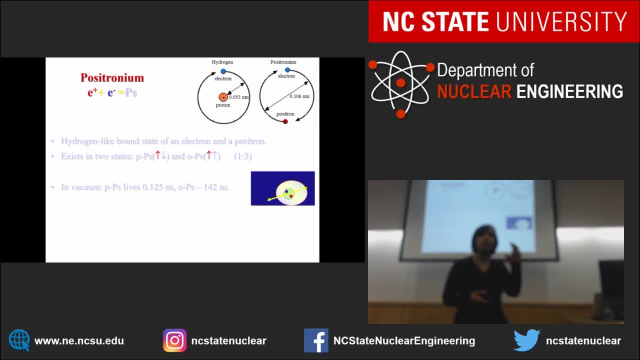 It's not the hydrogen atom, But what we call positronium. It's a study To understand a lot of stuff in quantum Electrodynamics And in physics. So it's a positronium atom. Okay, this is like. 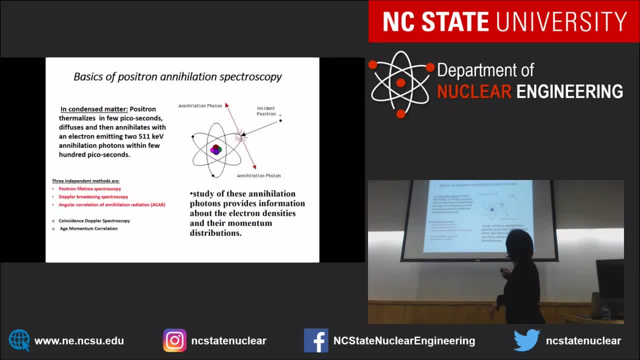 Really how they annihilate Together. So I just probably gonna skip this And it goes apart. People are interested in it And how positron use To look to the material probability And effect. It very much thermalize. It loses all it's energy. 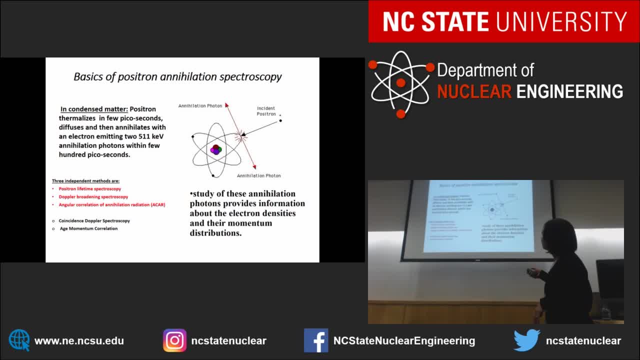 And it start, And then start to diffuse And then annihilate with the electron And emitting two photons. here, Like I told, every photon Has 511 kilo electron volt And we do different measurement. We look to how long The positron lived. 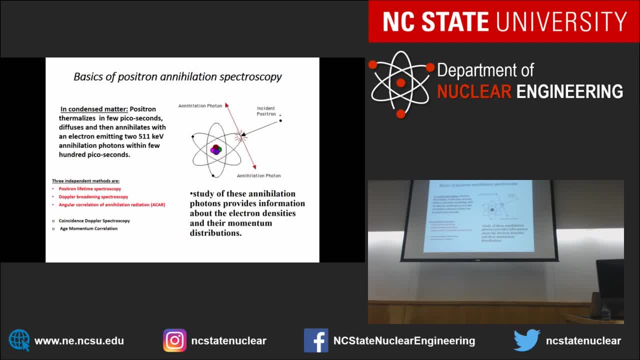 This one spectroscopy we can do And we can get some idea from this About the electron density Function of the material. Or we can look to the Energy Of the emitted photon, The energy distribution of the photon Or the angular distribution of the photon. 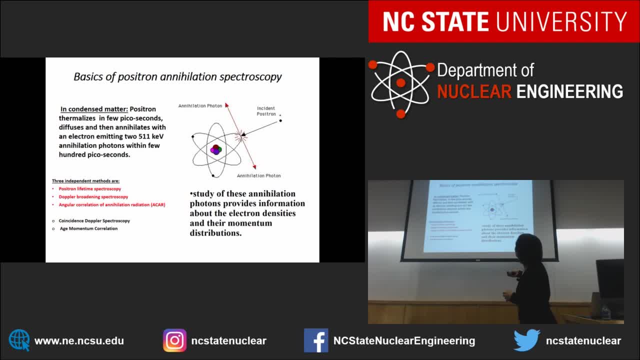 And we can really get a lot of important information. I will probably move to show you more work here. So this is why I said we have Three independent technique: Lifetime measurement, Duplar broadening spectroscopy Or angular correlation of the emitted radiation. 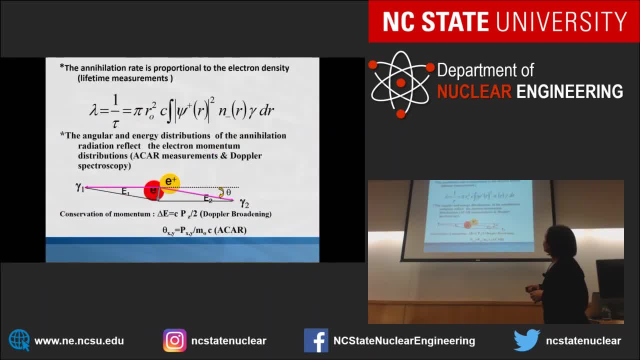 You can do So here for the Lifetime. So this is very much what I'm showing here. The positron wave function: This is the electron density function And how long the positron live It depends on the overlap Between them. 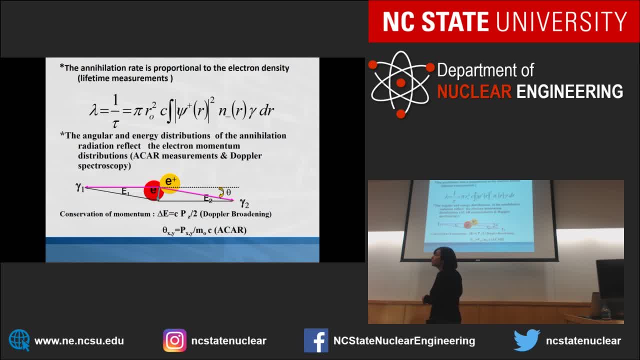 And very much. simply, I can measure How much the positron live And from this information I can get Information about the electron density function. This is how we can use: Measure the electron density function And then, from the Duplar, broadening. 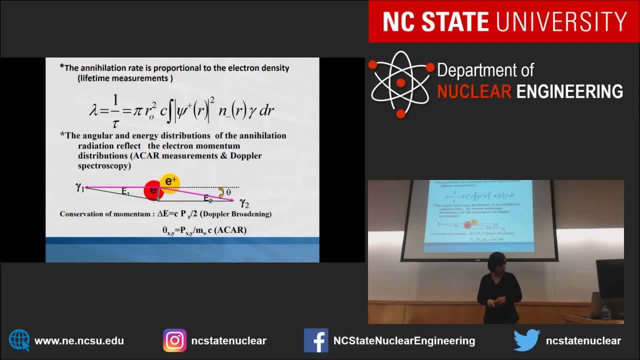 So if you think again about an electron And positron, If you have, electron has zero energy, Positron has zero energy When they annihilate, The momentum has to be conserved And the momentum energy has to be conserved. 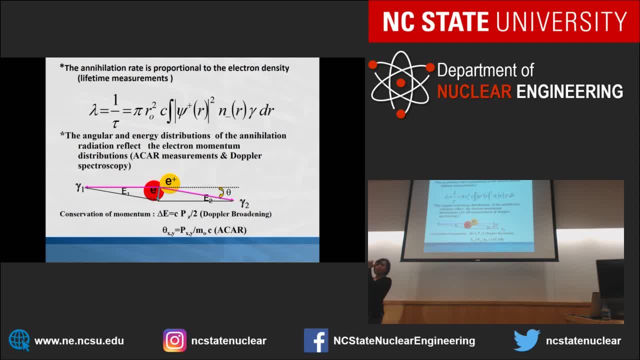 And to have to be conserved, They have to annihilate back to back. So they have to emit Two photon back to back. Each one has exactly 511 kilo electron volt For conservation of momentum to be right, And positron. 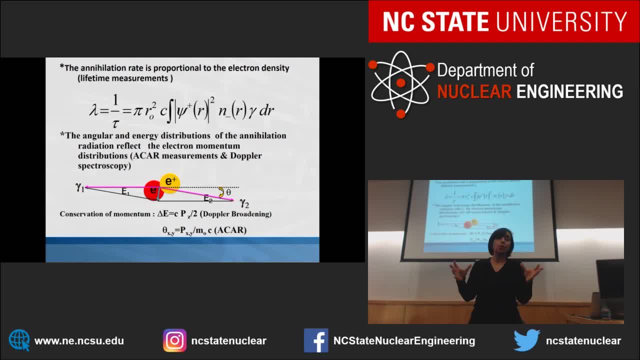 Already loses all it's energy Before annihilation, So it already doesn't have energy. But what about our momentum? What about the electron? Electron inside the material has momentum, And this is why We don't get exactly 511 photon. 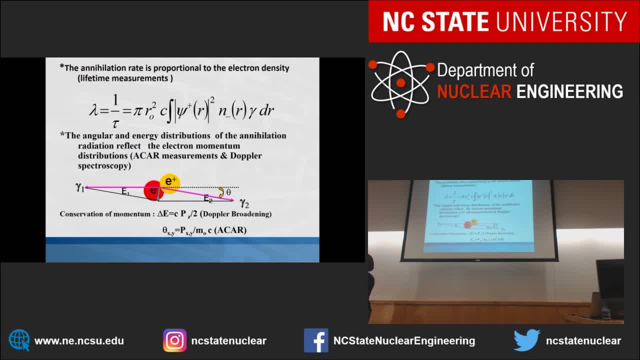 But we get 511 plus or minus Depending on the momentum of the electron. So the electron moving towards the detector, We get 511 plus. Of the electron moving away from the detector, We get 511 minus. And I can get this. 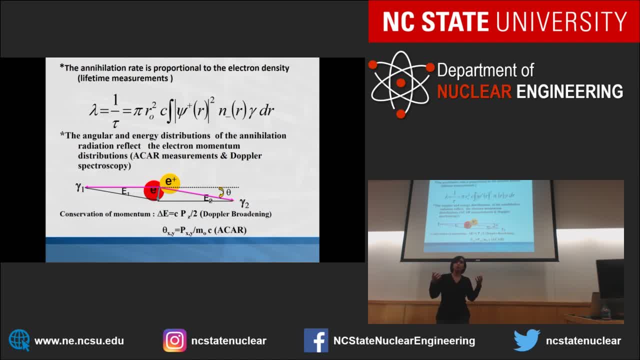 And just by looking to this I can get the electron momentum distribution In one direction of this. Why is this important? I mean all the probability of the material It based on the electron state. It really depend on the Electron momentum. 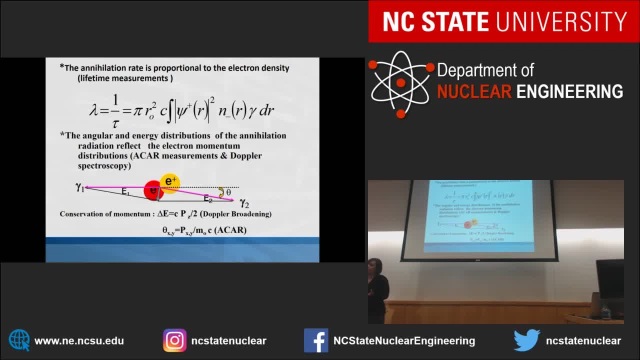 Of this electron. So for us to really understand the electron, The probability of the material, It's important for us to look to this. So this is a way we can measure by the energy, From measuring the energy of the Annihilation radiation. 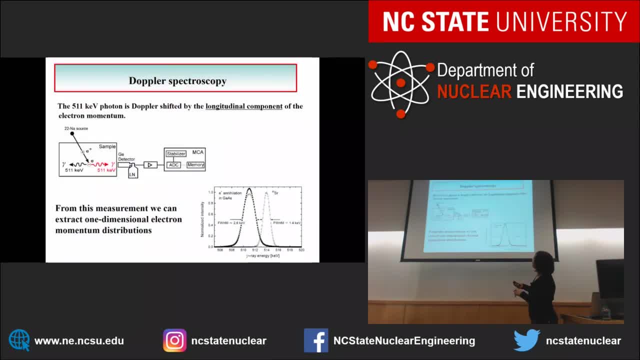 We can get this idea If we do. This is what I probably explained it already Before I show you this- That the 511 photon Is duplar, shifted by the Lentiginal component of the electron, And this is what I measure. 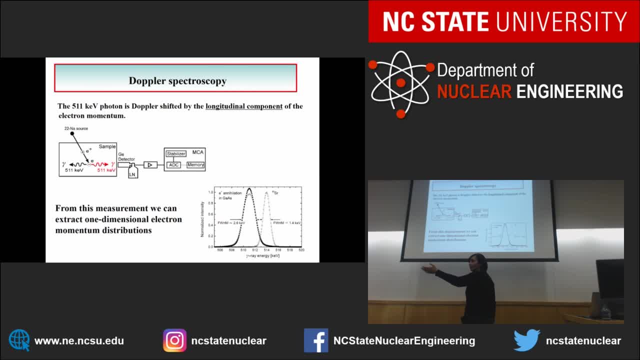 By doing here. If you visit the nuclear reactor facility And see the positron beams they have, So they have this detector. You see the detector here Which measures the 511 photon, The energy of the 511 photon, And you can get this. 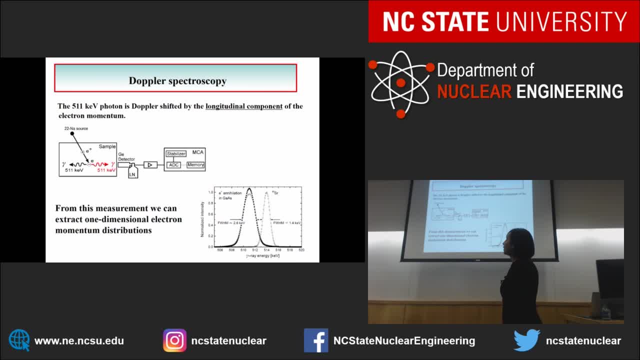 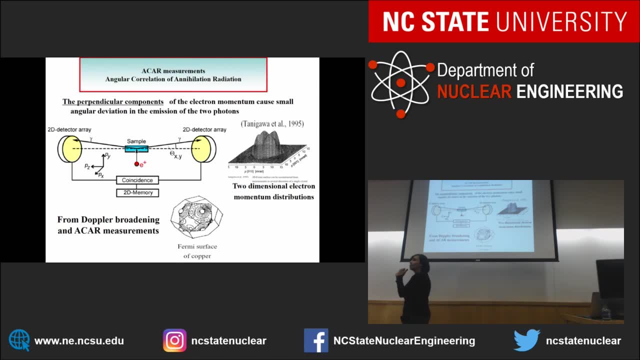 Energy distribution, From which you can get the momentum distribution Of electron in one direction. Then if you look to the, The transverse component Of the electron, What they lead it? They lead to the photon emission And in the xy direction, 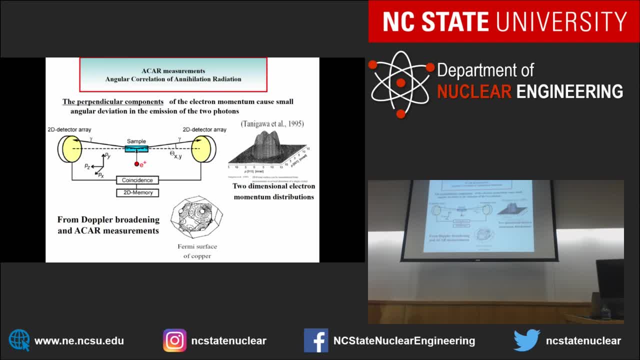 So very much is the electron momentum. Instead, if you get Two electron exactly To back, You get plus or minus It based on the transverse momentum Of the electron And from this you can measure the Electron momentum in the x direction. 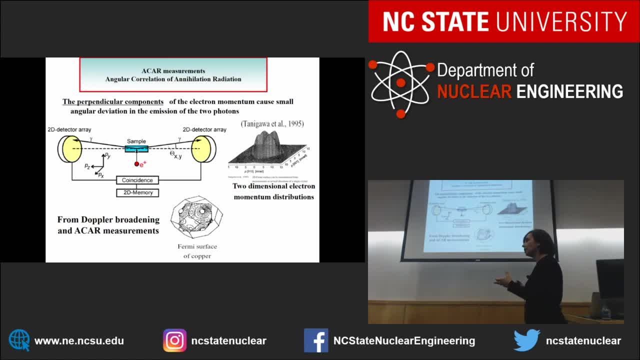 And in the y direction. And people in the past have combined The duplar broadening measurement And what we call here The angular radiation, The angular correlation Of the annihilation radiation. They call it ACAR And they determine: 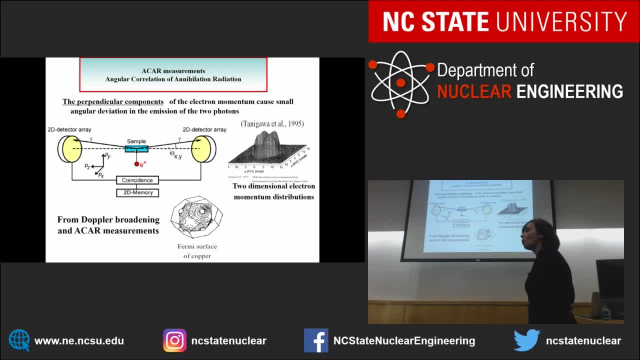 The full electron momentum, Distribution of the electron, Or what we call Fermi surface. You hear about this word. I mean a physicist like this very much. It's very important for us To really understand any metal Or semiconductor or oxide. 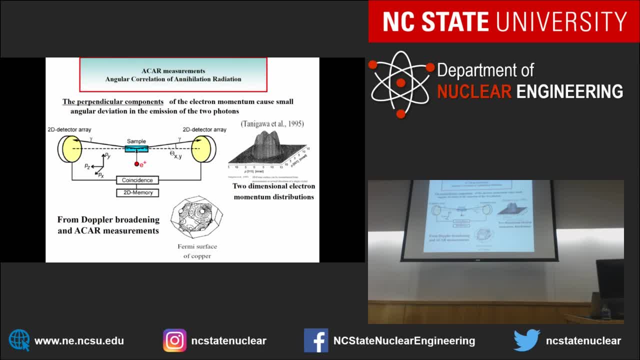 We look to the electronic structure And the Fermi surface of this material. How we measure this stuff? We measure- one of them, of course, Is the positron annihilation spectroscopy- How positron has been used To determine the electronic structure. 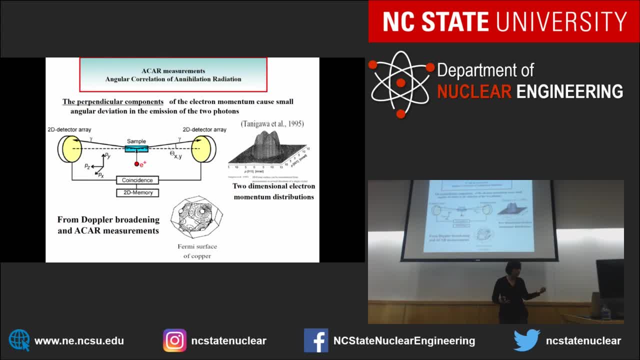 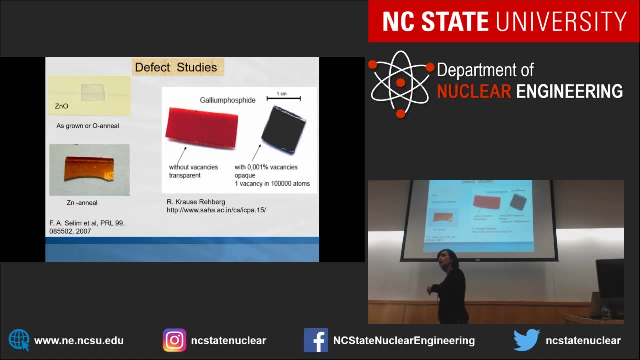 Of material And, up to now, If we develop new nano material or something, We can apply positron annihilation To do this kind of studies. Okay, Now I'm going to talk about The important part of now. People use positron. 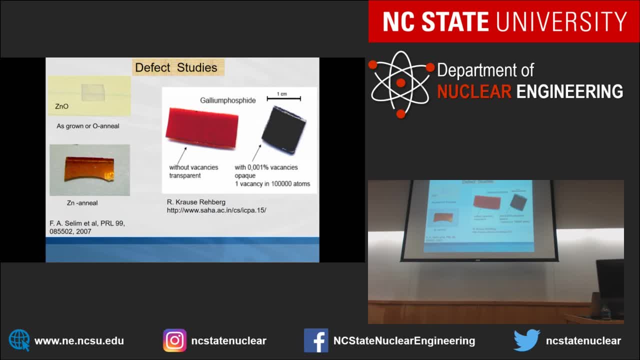 Is to look to defect For you. You look to defect In irradiated material. It's important for you. You want to understand defect, Because defect and damage from material And it's something bad Right, You really want to avoid this. 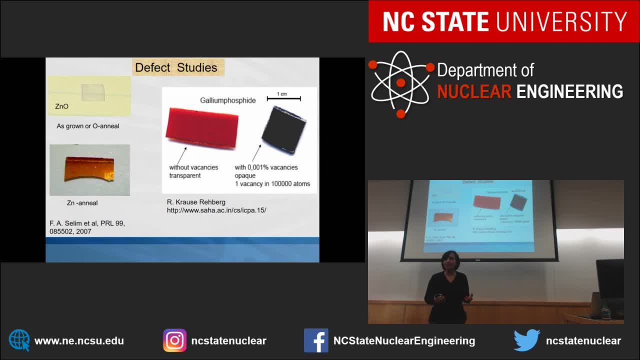 But this is not all the story of defect. In fact, for us People who work in physics and material science, Defect is also very important, But it's not the bad part, It is the interesting part for us. So defect really for us, is important. 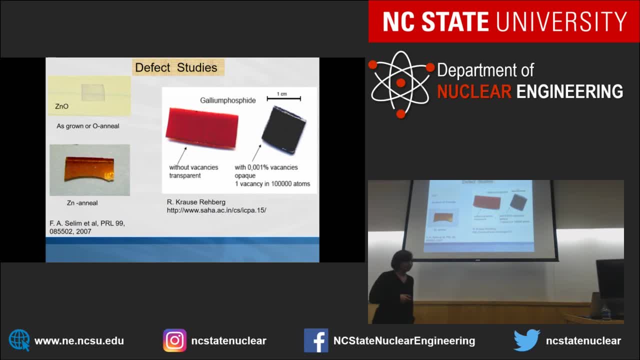 To manipulate the material properties. So When I started I told them: You're going to study defect Or just defect. Defect is important. This is what determines the electronic properties of material. So let me give you some example here. 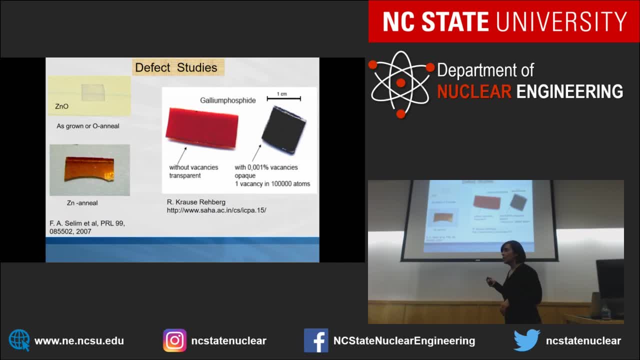 This is gallium phosphide. It's a semiconductor material. This is how it looks. It's transparent And it looks like this color. It doesn't have any defect. Here we created vacancy in the material. How much we created Zero. 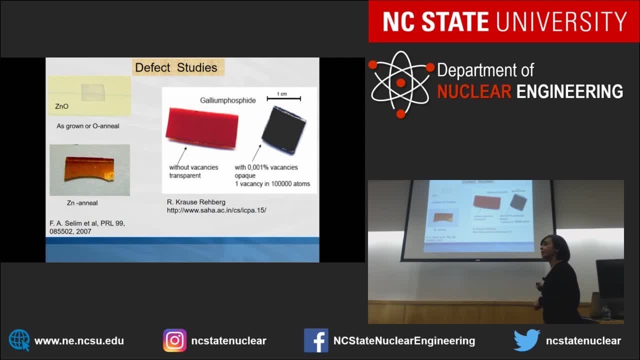 One percentage. So in every 100,000 atoms Are created vacancy. You see what happened to material. It's become opaque. The optical properties of the material completely change. This is another semiconductor material Important here: Zinc oxide, And we grow this stuff in our lab. 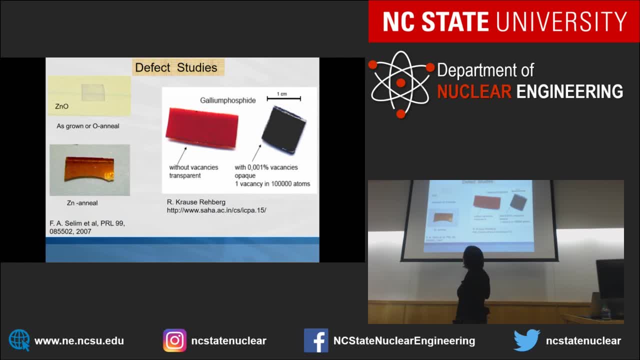 Zinc oxide Single crystal. It's transparent material. We anneal it here in zinc vapor. It becomes red And the electrical conductivity becomes very conductive. We include the conductive several times higher than the original conductive. What I'm telling you? 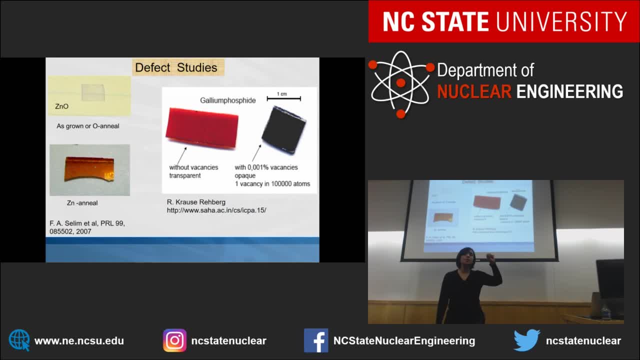 Because always when I introduce this to my students, I tell them: So this is really to understand how defect is important For people who work in the area of semiconductor And electronic Or photonic, Because we use defect to manipulate the material. 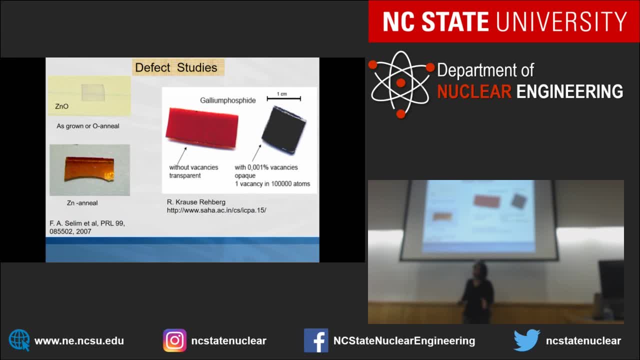 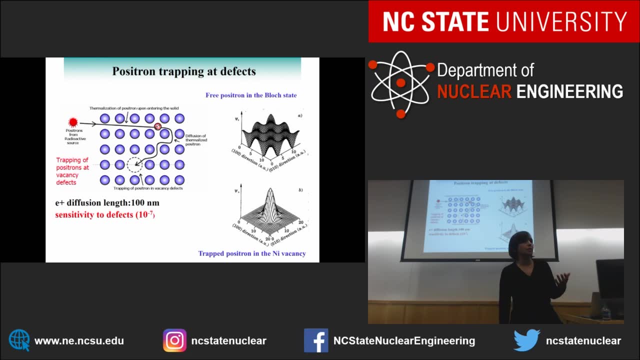 To create interesting phenomena. So this is really how defect is important For damage stuff, But in general, Okay. So why positron? How positron get to look to defect, And I also want to show that it's unique technique In this sense. 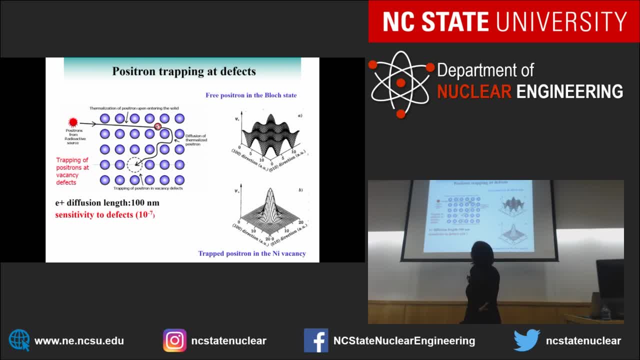 So positron here? Assume we have a positron from radioactive source Or from BM, Wherever you get it, It enters the material. It always thermalize very fast Because the annihilation in flight, The cross section, is very low. 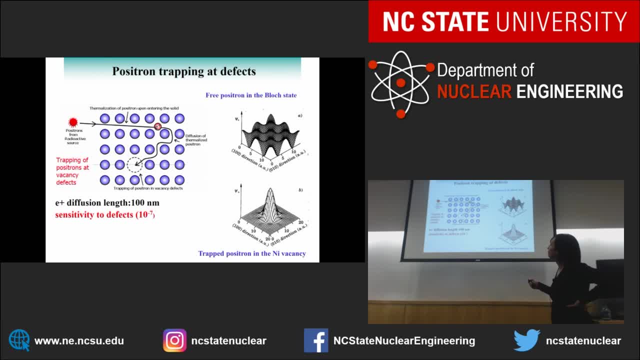 So it thermalize very fast To lose it's all it's energy. And then What it does? It start to diffuse As a particle without energy inside the material As soon as I find A vacancy Or any opening Even smaller than the atom. 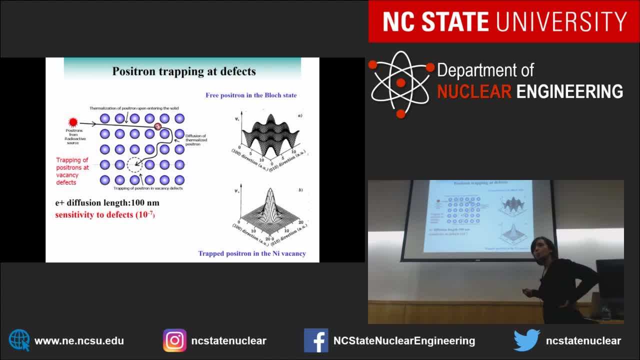 It get trapped there. And why this? You understand why? Because positron is a charged particle, All the nuclei here. So the charged, The nuclei is a charged particle, The positron is a charged particle, So there is a repulsive force. 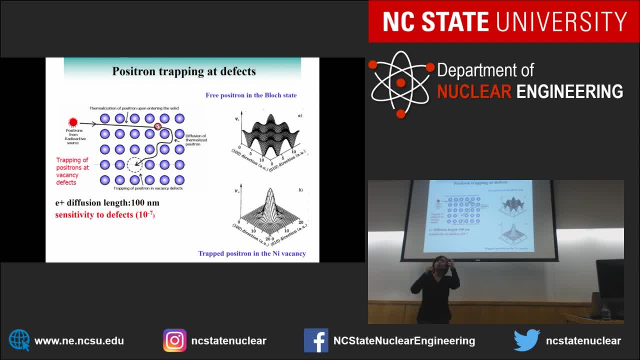 Right, They try to be away. So the positron try to be away from the nuclei, Which is a positive charge, So it really never come closer. It always go through this Opening area in the crystal, But this area it doesn't have. 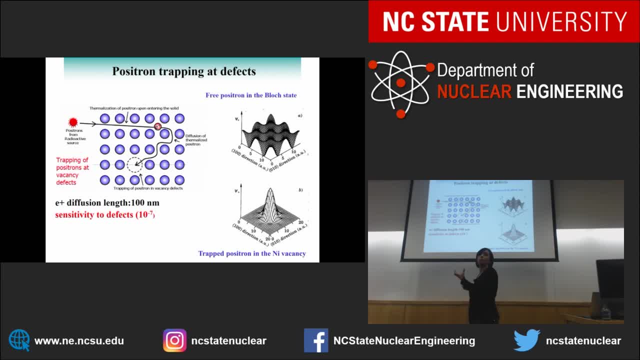 The charged particle. So it form a minimum potential for positron. Everywhere else There is repulsive force. It makes the positron to stay away, But this one attract, The positron here attract. This is really how positron can look to. 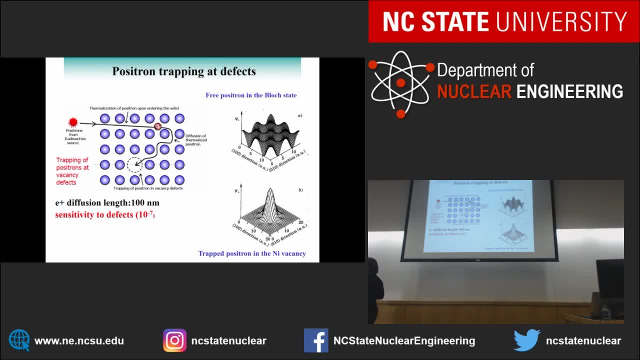 Very, very small vacancy: Single atom missing, Or it can, Even if you have, like some Less than single atom, Some opening between The plane or something. Positron can Prop this. The difference, The fusion length of positron. 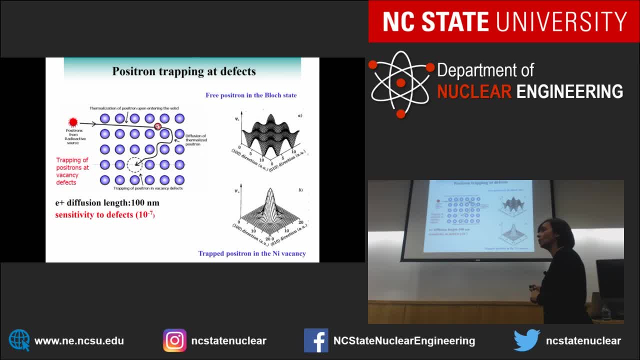 Is very long. This is really very long compared to other particle. It's 100 nanometer. What's that mean? In 100 nanometer You can probe about 10 to the 7 atom. So if he find One atom missing, 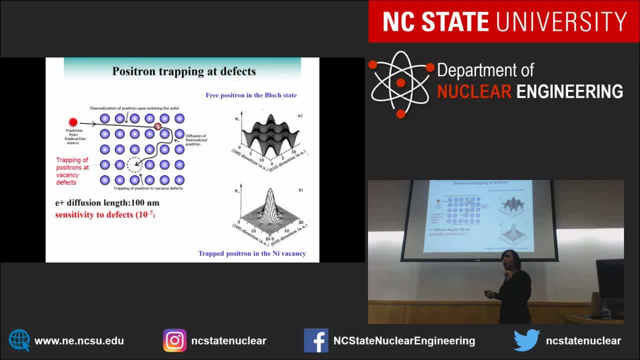 In 10 to the 7 atom. It can get trapped here And it trapped in chill analyte. So we talk about here Probe with a sensitivity 10 to the minus 7. And it can see defect or vacancies In term of atomic size. 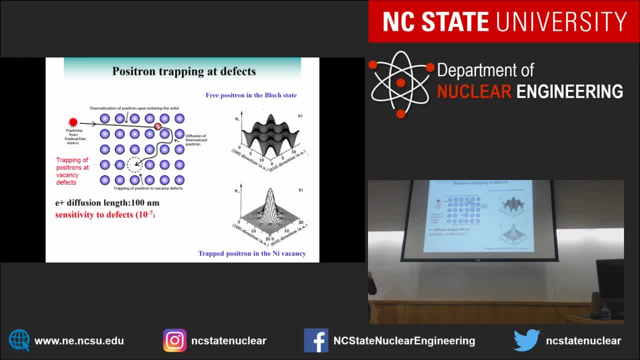 There is no other technique can do this, So high resolution transmission Electron microscopy. They can not see this kind of defect And they don't have this kind of resolution. This is really why we consider Positron halation spectroscopy. 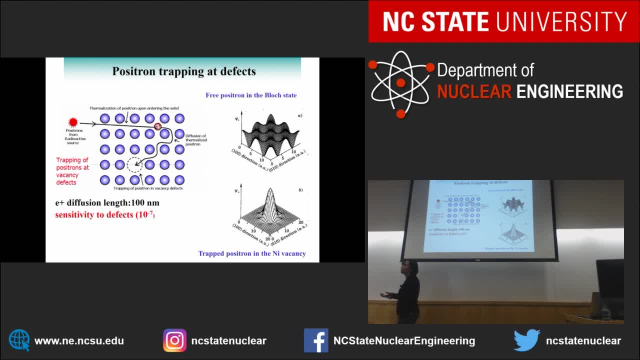 Is a very, very important And effective probe To look to this kind of stuff. This is here, Probably, This is always, You know, If you study quantum mechanics And you know This is a positron wave function In a block state. 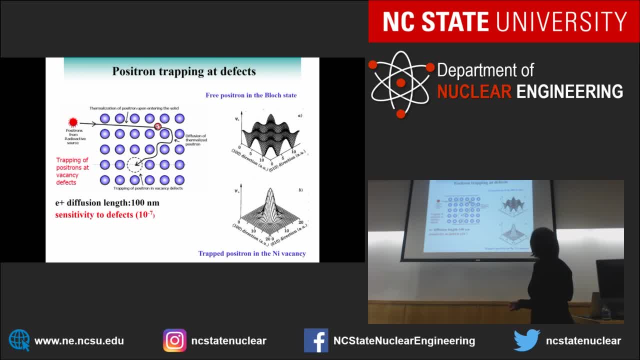 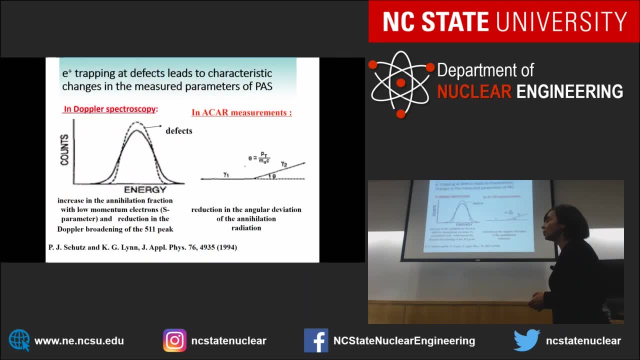 In the bulk material without any effect. We call it block state Here. if the positron get trapped in a vacancy. This is a positron wave function Looks like this- Not spread in the material. So what happen when the positron get trapped? 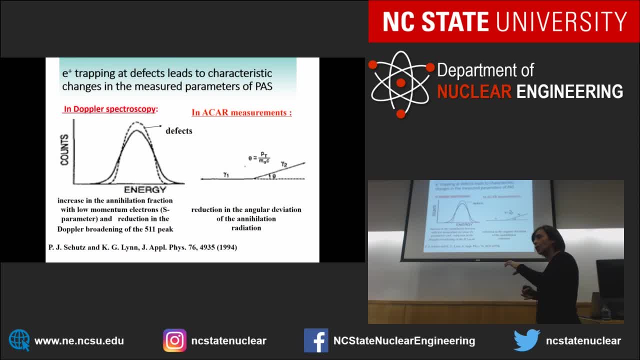 It analyte And we see this trapping And the positron halation parameter we measure, And this is how we can really know What we have, What kind of defect we have. So here, for example, In Doppler spectroscopy, 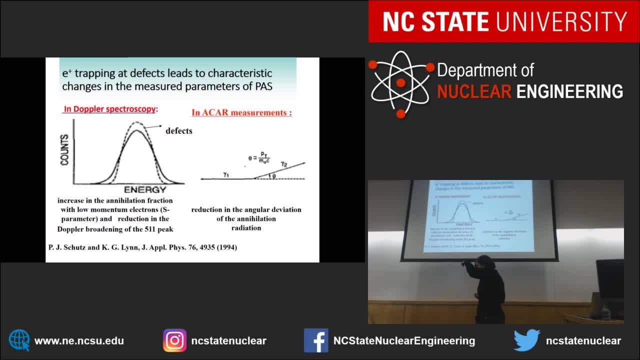 When I told you Doppler spectroscopy very much. We measure the 511 peak And we can see that, the peak of the 511. The energy: We measure the energy of the 511. The annihilation radiation of the 511. 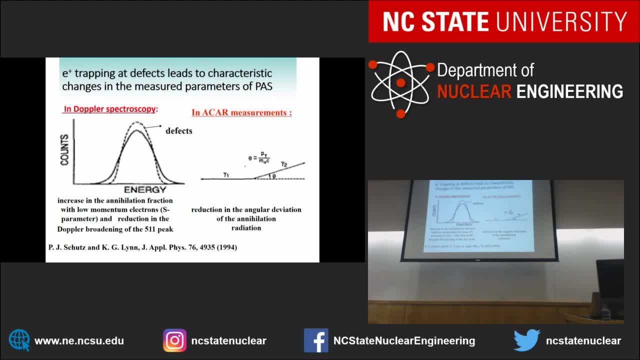 We have to do high energy resolution measurement, Very high energy resolution detector, Like many of detectors- Probably people familiar with this here- And we use this kind of stuff. So the peak of the 511. Is Doppler providing by the electron momentum. 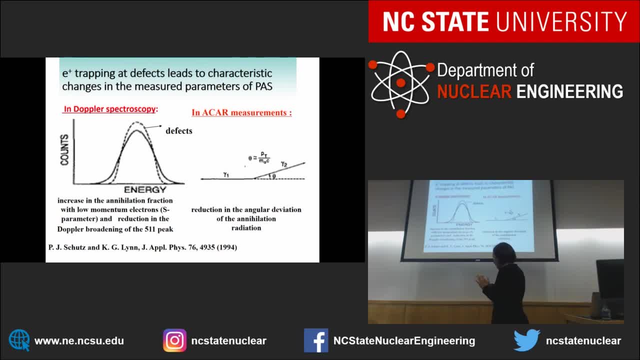 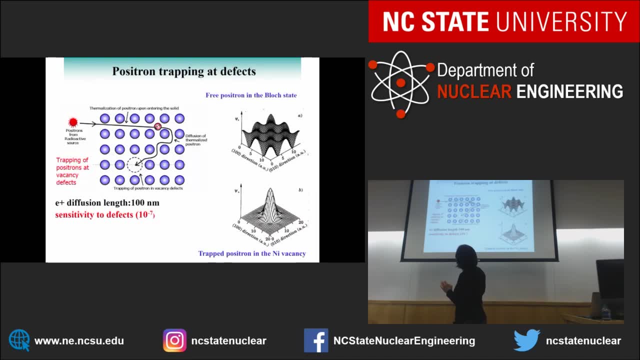 But if you get The electron trapped In a peak here, If you get the electron Trapped in a vacancy, What happen? It is going to annihilate, mainly with the valence electron, Because it only sees the valence electron here. 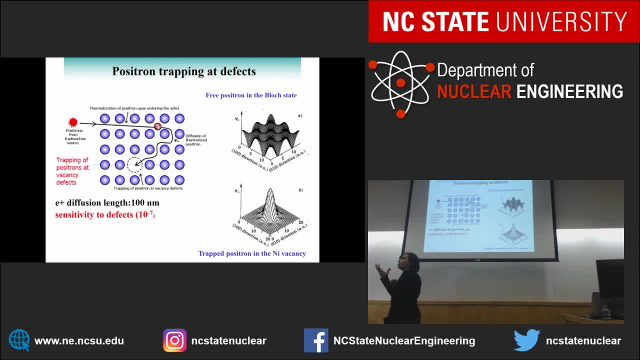 It doesn't see the core electron. You know the difference between The valence electron and core electron. Valence electron has lower momentum, So you get the narrow peak, The 511 peak. It's become narrow And very much we can measure. 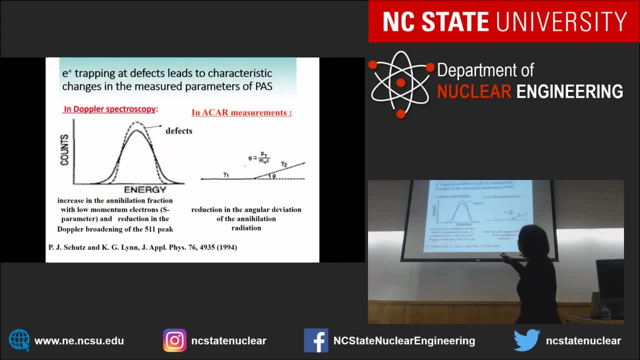 What we call from the 511 peak We can measure here. You see the peak here become narrow. If I have defect. Now here is Doppler recording This here. Doppler recording become less And very much I can measure The ratio of positron annihilation. 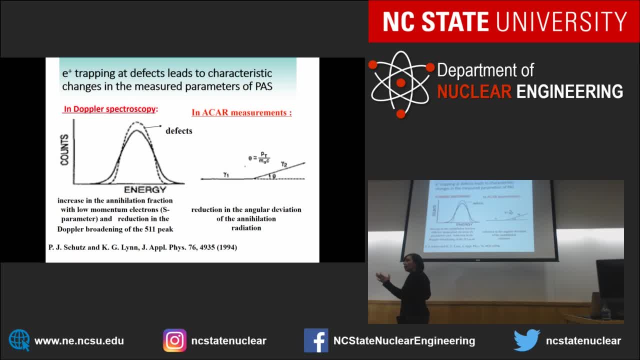 Compared to the ratio annihilation With core electron, And I can use this to give me an idea about How much is that defect Increase by doing this. And of course we can do it also this If we do angular deviation. This is not common technique. 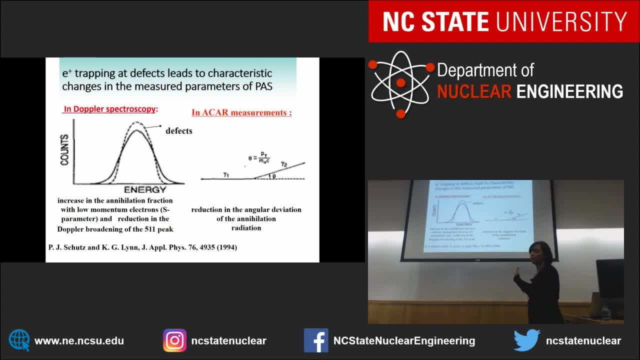 People don't use it too much For this specific to look to defect. Why? Because it's a very expensive technique. It need lab, Very, very, very large lab to do this. This is very much. I said how we can Calculate the annihilation with valence electron. 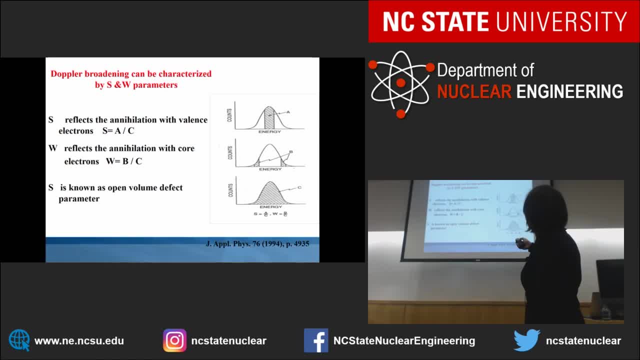 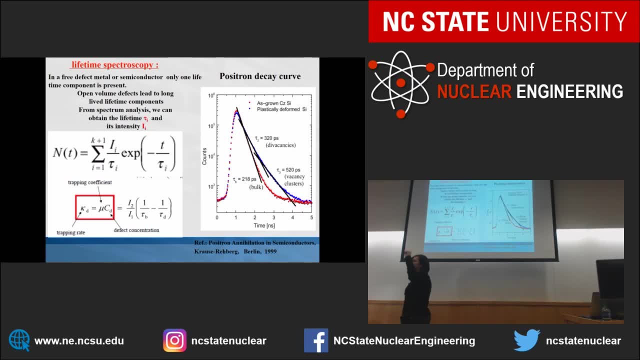 The annihilation with core electron. Let me move to this one, Which is the lifetime spectroscopy. So When the positron get trapped In the vacancy, What's gonna happen In the vacancy? It's very much has low. There is no material there. 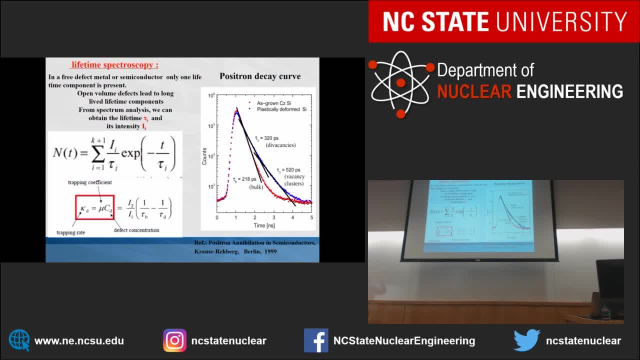 So there is electron surrounding it, But the electron density in this area much less. So what they expected for the positron, It's gonna live longer. So positron in most material, For example in most metal and semiconductor It made about. 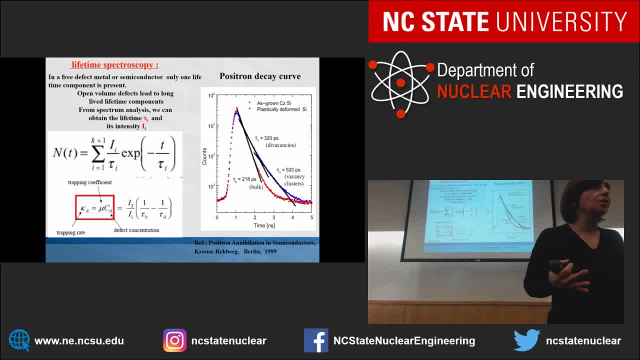 100 picosecond, 200 picosecond. This is the life the positron live. But if I get trapped in this defect, It's gonna live longer Because of the Lack of the electron here, Of the electron density become less. 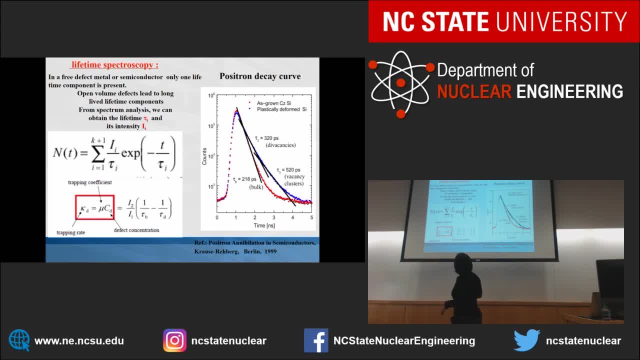 So it's gonna live longer. So if you look here What we can do, We can measure this Much. we measure exactly how the positron. It should be very high timing resolution, Because we're interested to measure something in Few hundred picosecond. 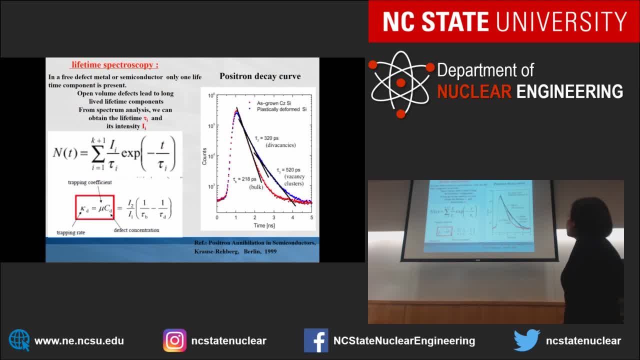 So we measure this And from this curve We can see the decay constant. We can share the How much the positron live And the lifetime is related to the Size of defect. So I can determine from this measurement If I have single vacancy. 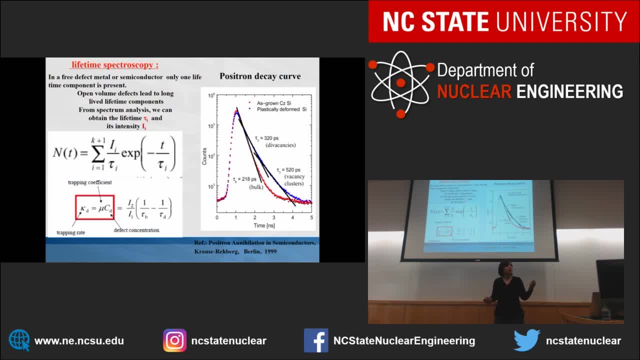 If I have double vacancy, If I have cluster, If I have dislocation, And from the intensity of this component It's also related to the Intensity of this kind of defect. So if you look here, What we have This is silicon, for example. 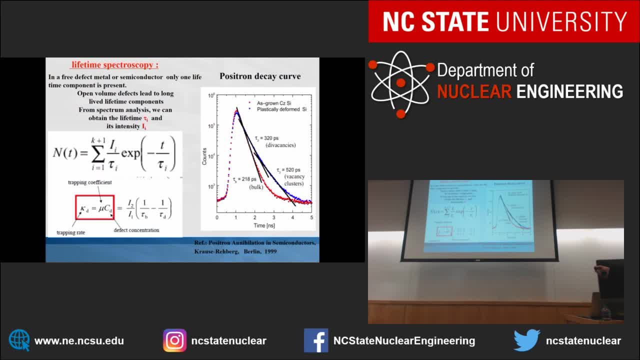 Silicon without defect will only live Measure one lifetime component with the bulk. But if you have silicon with Defect Vacancy cluster We measure three component: From the lifetime- here We can determine what kind of defect, And from the intensity. 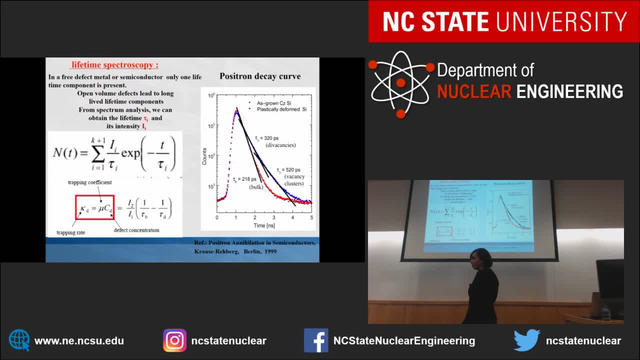 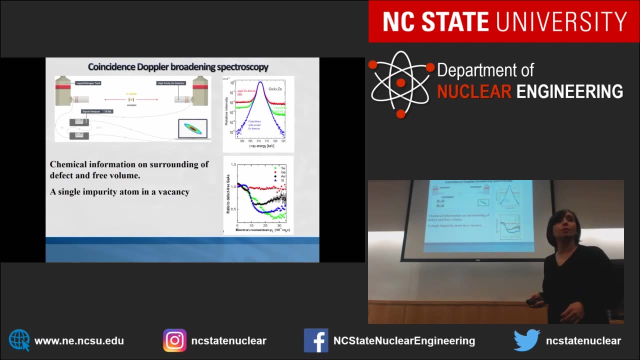 Of the component, We can determine the concentration of defect. So this is why we consider Especially. lifetime is really important, Because it can tell us This information, Something also we can do. People are not really very familiar with this, But this is some of the important stuff. 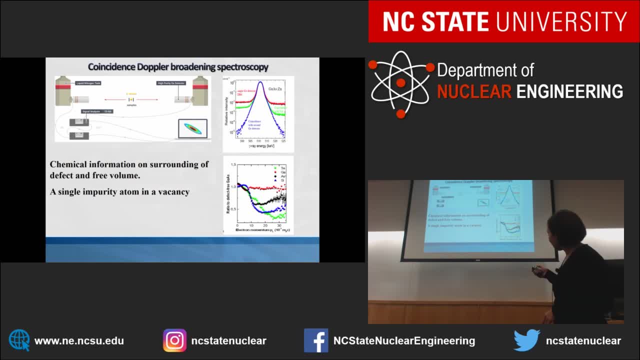 For positron And how can we measure the Identity around the defect? Do you know What surrounding is the vacancy, Or if you have atom Trapped like some impurity In this vacancy? Can we measure this? In this case we do. 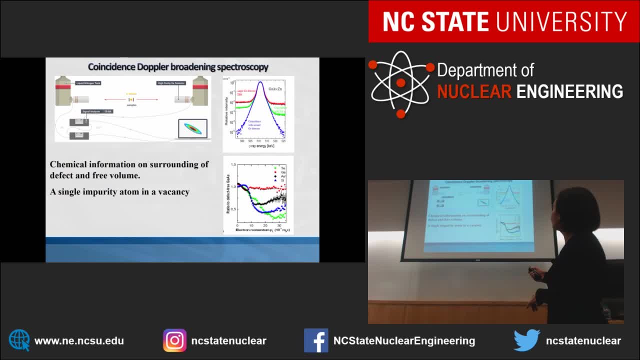 So we measure the 511 peak By two detector Like this. So instead in single detector You get this is a 511.. You see high background radiation, But if I use two detector This is very clean Spectrum here. So you see, this is very clean. 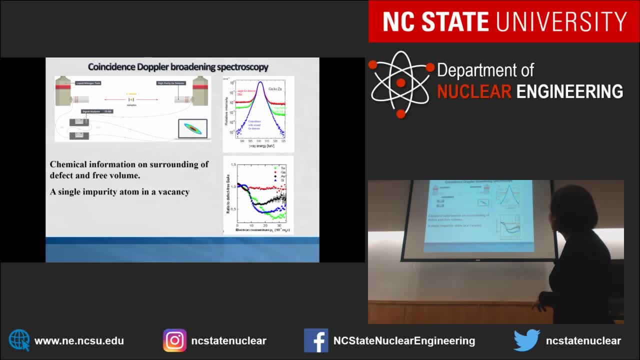 The background become very low Almost. I improve it 10 to the 5. The factor: Why is this important for us? Because in this part I can see positron radiation With core electron, So we can show here This is what we call the electron momentum. 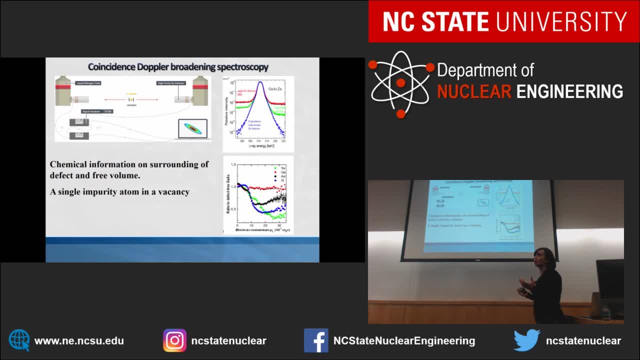 And the ratio curve, Each one of these corresponding to certain element. Why? Because in this case I am measuring the material Valence electron. They are affected by the crystal field in general, But core electron They are actually only They retain the chemical identity of the element. 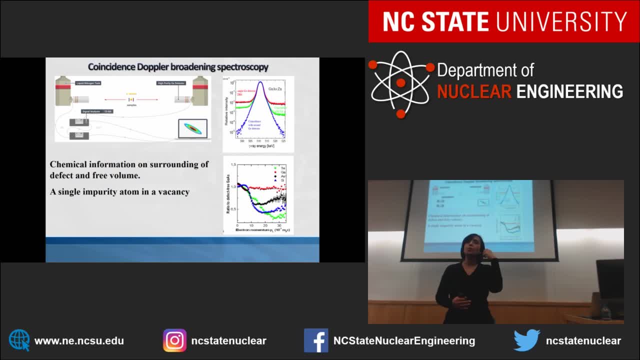 So they are not affected. So when positron Annihilate with the core electron, I can know what kind of element Surrounding the defect. I'm not measure, I don't care about impurity, general material Like other technique. 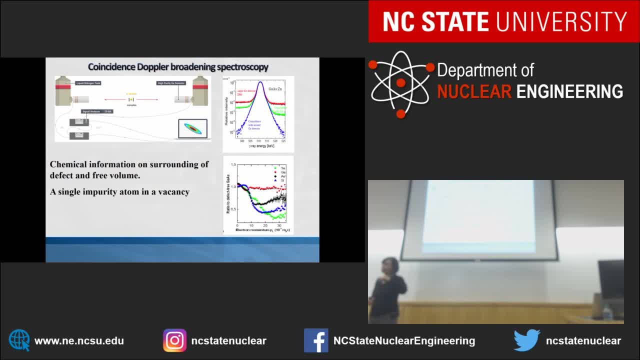 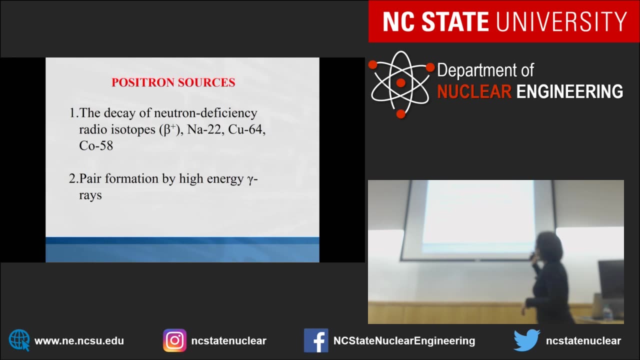 The impurities inside the Vacancy Or the surrounding the vacancy. And this is, of course, has Probably people who work in nuclear material. They know this is really quite important To understand the material And their behavior. Okay, So this is very much what the positron. 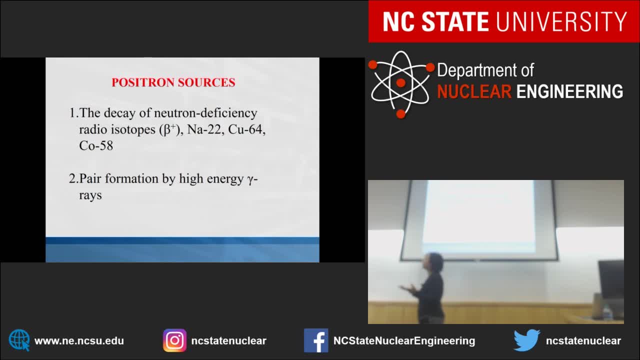 I hope you get some idea how positron work In term of looking to defect. So positron source available. We can get Regioactive source. We can get positron, But they give positron with a Wide energy range. 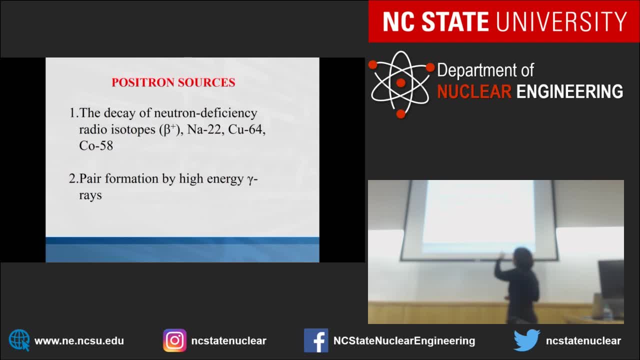 Other thing We can generate positron From bare production Is the opposite process for Positron annihilation. Positron annihilation: you have electron, Two particles. they annihilate Bare production. you have the electron positron. They actually 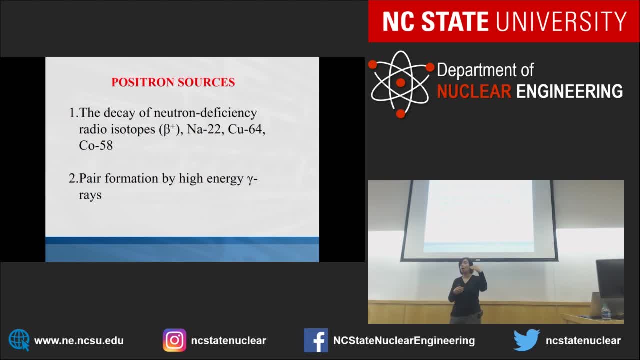 You have a gamma rays With high energy Above 1.02 MeV. What happened for this high energy? It can give two particles: It can give electron And positron. And this is the way how you generate electron, How you get this high energy. 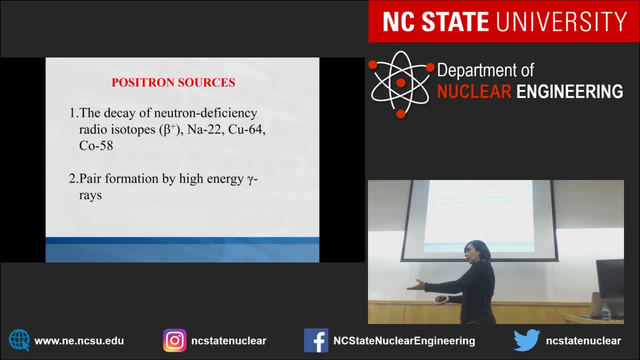 You get this high energy from electron accelerator Or you get it from neutron reactor Like what you do downstairs here. You have like a neutron beam And you have a cadmium source. It gives you the high energy- gamma ray- And then through the pair production process. 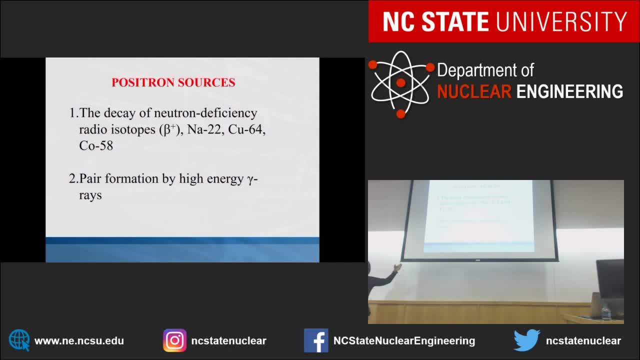 You get the positron and positron And you get the positron from it. So the sodium 22 is naturally A positron emitter. Yes, You have to irradiate it, In fact Also the sodium 22.. They prepare it also. 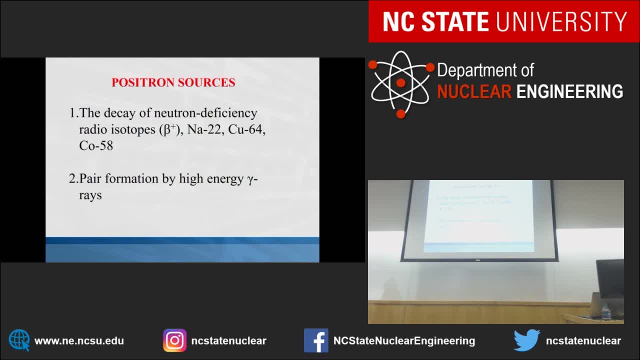 It's palliation source too. Exactly, you have to do it this way, But they prepare it, For example sodium 22.. They do it as palliation source, But they give us radioactive, So we can use it for this sense. The copper 64.. 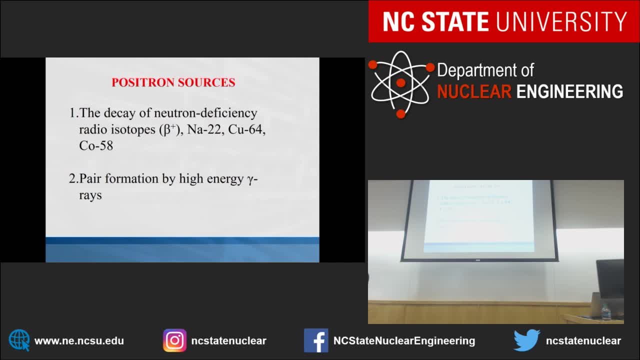 It's actually very short, So they use it for us For hours actually, And the same stuff they use for Positron emission tomography. It has to be very short lifetime. So this is the kind of stuff, So how we get positron. 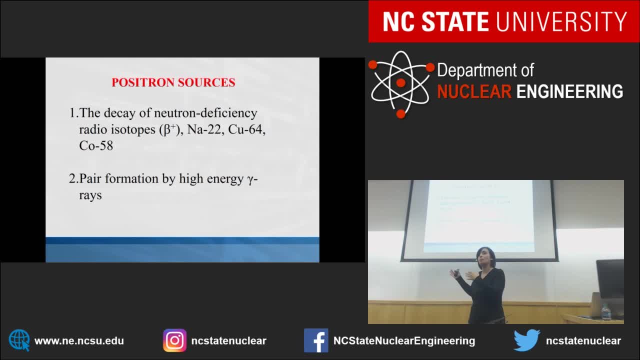 Of course, it's always with the issue. I talked about positron, By the way, As a positron spectroscopy for defect Positron could be very, very Nice tool If we do all of the stuff we do With electron, like electron diffraction. 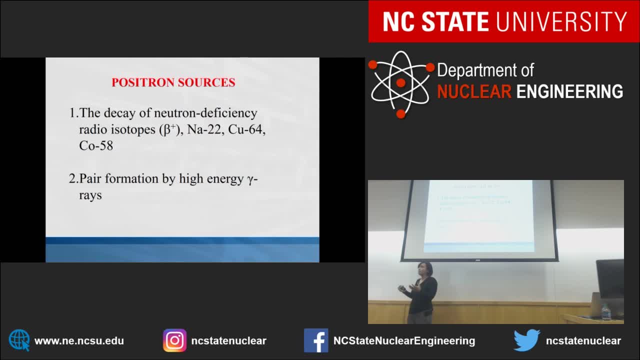 Positron microscopy. It's really. positron is going to be more clean. Why this stuff is not common? Because positron is antimatter. It's hard to keep it, It's harder to have it. So, having always, How much positron we can get in the wallet so far, 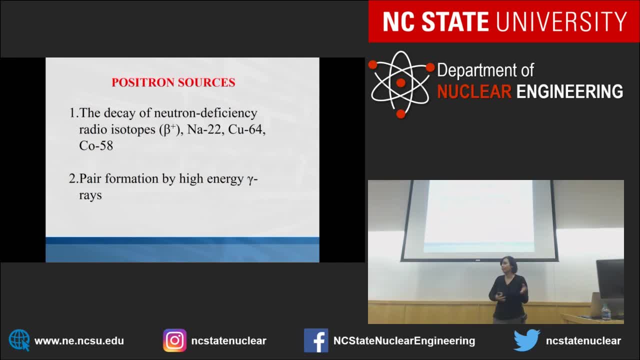 Maximum: 10 to the 8.. 10 to the 9 per second. If we get more than this, It's really interesting science. That actually better than we doing with electron, With electron as a product. So anyway, This is the conventional. 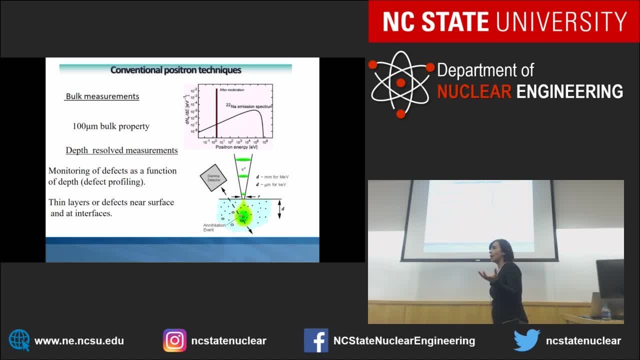 I talk about the source. So if I use the source right away, I can only do bulk measurement. You have bulk material And you have beam going through this bulk, So you give the Idea about the material As a bulk Because the positron coming from the source. 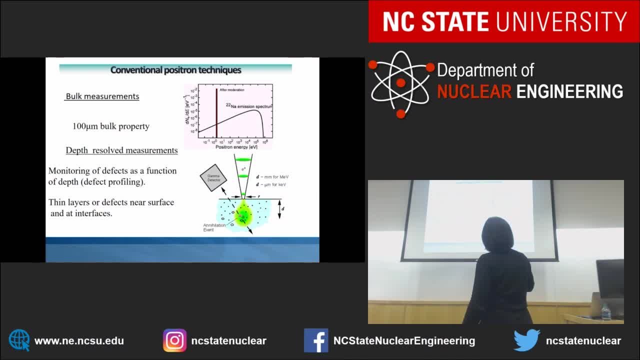 They always have energy like this. So the, For example, Sodium 22.. You see how wide of energy So I cannot measure. I'm going to measure the entire thickness of the material, So like several Several micron. But if I want to do, 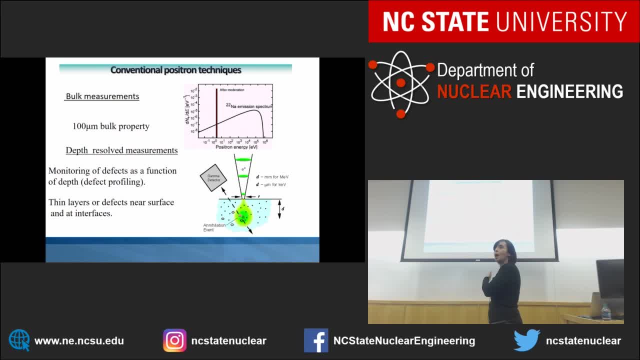 That's a resolvent measurement. I want to look to sand film or surface. I have to make a positron beam, So we have to moderate the positron And then start to accelerate Them to certain energy. So you have guys here. 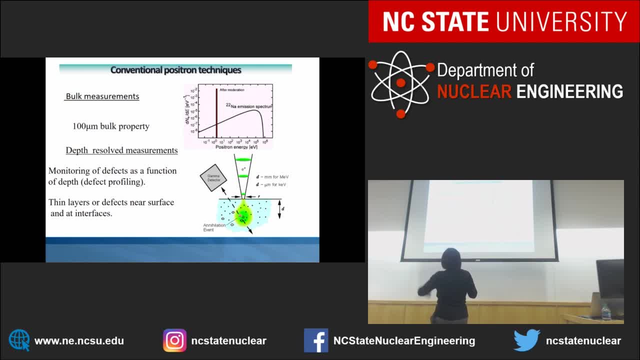 You have a positron beam That you can really look to that certain area, Certain depths in the material. So this has been, I think, in probably 1980.. And the Kelvin learn, by the way, Who, one of the people Who developed this technique. 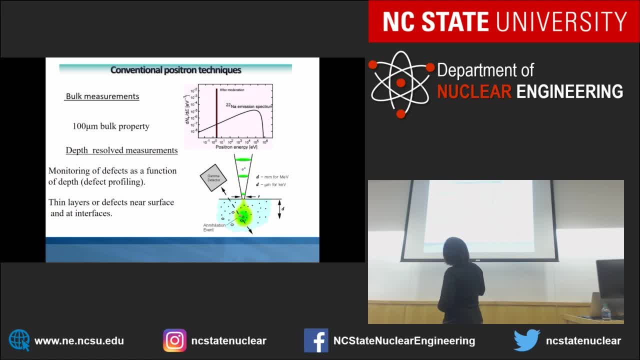 To develop positron beam, To do a positron beam, To do a resolvent measurement, Which monitoring of defect As a function of depths, Or, for people like us, We can send film and Interface. We need a beam. 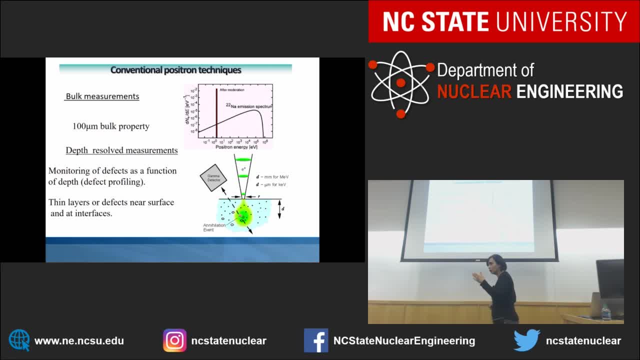 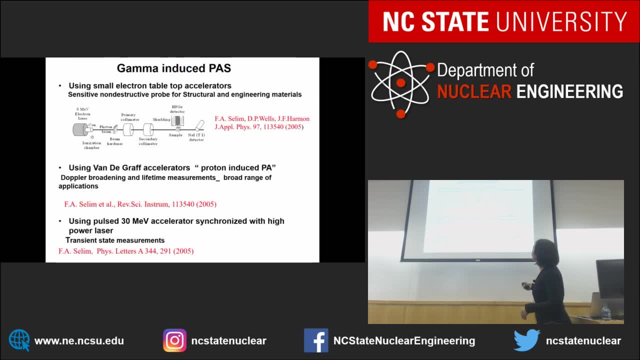 We cannot use bulk material. When you do ion radiation, also You need beam. You cannot use just bulk measurement. This is one of them That we mentioned, Because this is actually one of the. This is one of the. This is a technique. 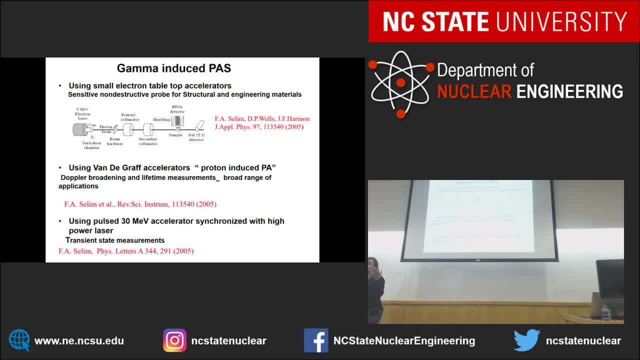 I started it and I invented it At the beginning of my career. I was a positron source like sodium 22.. Or per production, What we actually were doing here. Instead of doing this, I just use gamma ray directly And don't generate any positron. 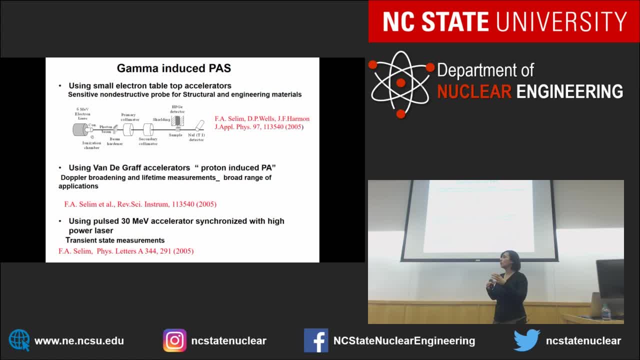 And I just expose the material to gamma ray And I use positron annihilation. So all the process It happen inside the material And we call this gamma induced Positron spectroscopy. Why this is important technique for us? Because we don't have to go through all the hassle. 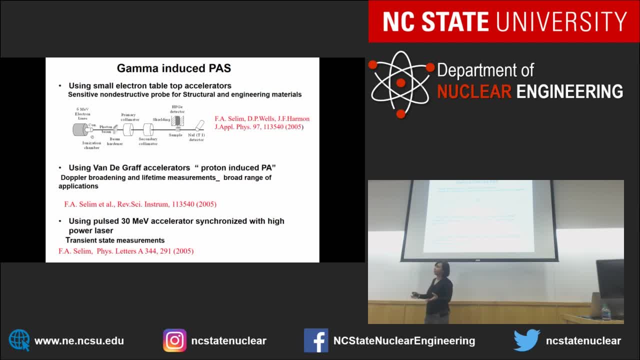 To generate the positron Or to generate radioactive material. All I have, I have the gamma ray And then expose the material to it And then I can do lifetime Or duplar spectroscopy. Of course there is several techniques. We use several accelerators. 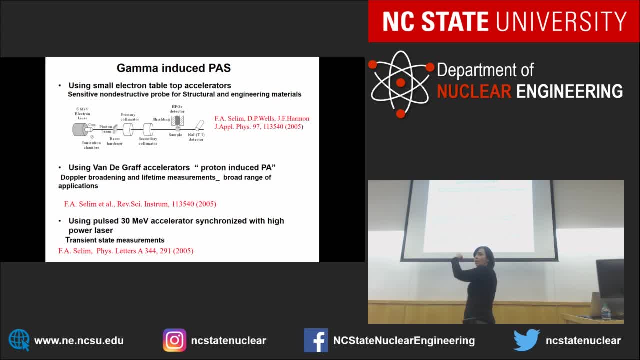 To be able to do this stuff. But also interesting in something, Because gamma ray is very penetrating, So you can go to very high depths With positron beam. You are also limited to very thin layer, One micron. But if you want to really 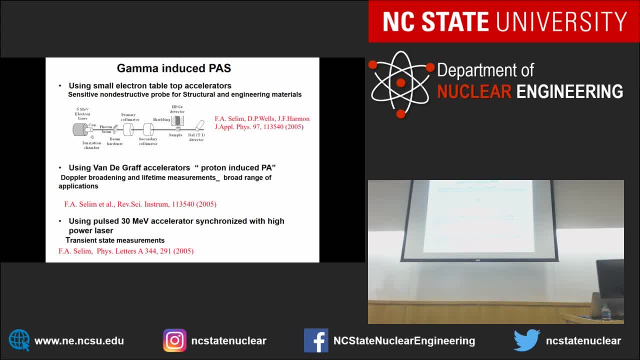 Drop something like Centimeter Or millimeter stuff. We don't have a technique for this- And even all the methods you use- X-ray or electron microscopy- All of the stuff for very thin material. So if you want a technique for 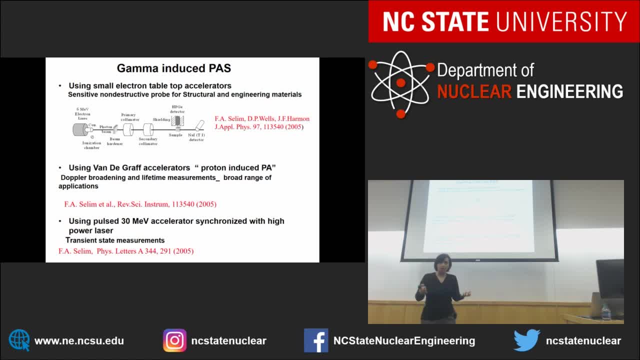 Very thick material. What's our option? Ultrasonic stuff, But they are not sensitive. They become sensitive after you get crack in the material. So if we develop positron, Which is a high sensitivity unit To be able To look to very thick material, 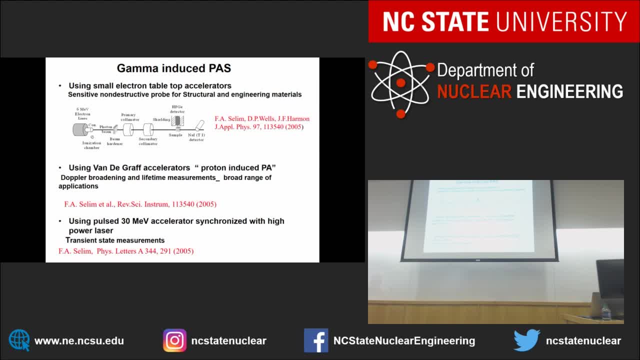 This is kind of interesting technique. So in fact I developed this technique in Idaho And I've been using it, But then I left Idaho And it's never been. But German people actually took it And they developed very nice facility On their superconducting accelerator. 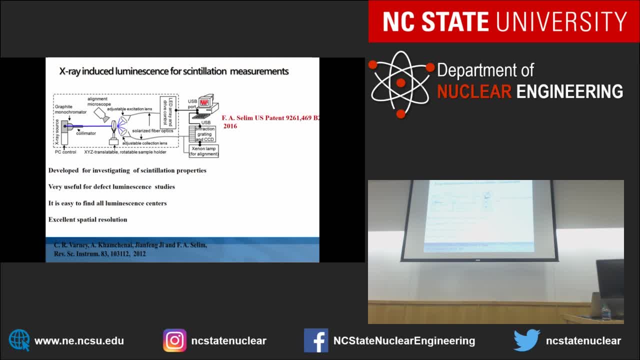 change it. We can use any source here. Is it one that's? the target is replaceable? Yeah, I mean the tube itself We can replaceable. yeah, Yeah, you can go to higher, to higher one. So let me actually show you here what's really interesting, especially regarding 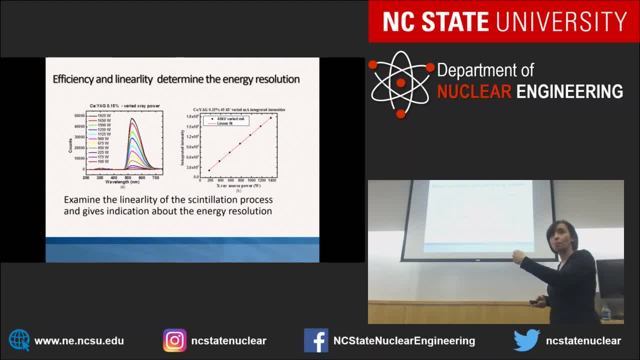 the, because I said this is important for the centralization properties of the material. So you can see here, when we change the, when we change the X-ray current, so we change here the power from 100 watts to 170 watts, So what you can see here we can really change the emission and then we can. 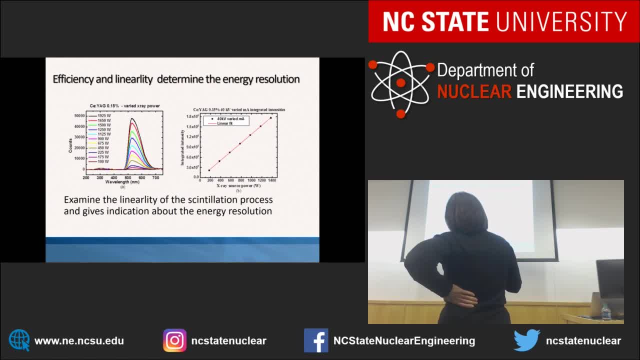 take, integrate the intensity and if you can see the luminescent intensity versus the X-ray power. And what's interesting here, because if it give me linear, this mean this material could work for me good material as a centralization detector because it has linear response to the effect of X-ray. 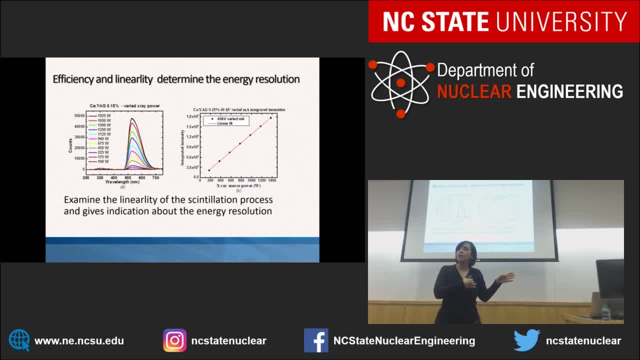 So if I increase X-ray power or if I increase X-ray current as well as the X-ray current as very much I see, you see this is linear. So this is really good. It tell me a really important thing about the linearity of the centralization. 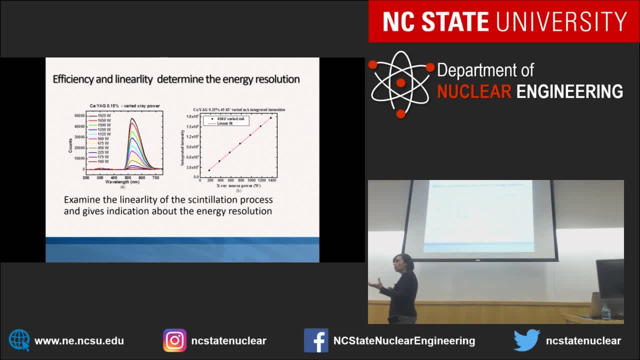 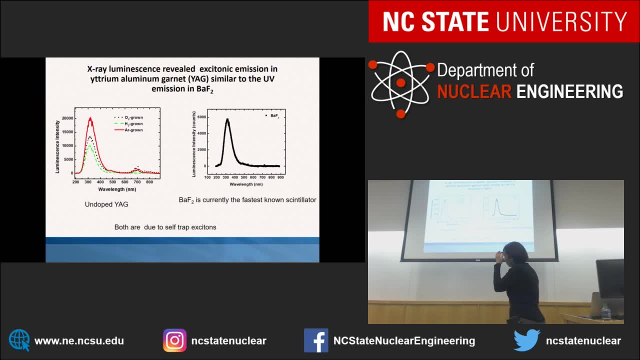 material developed. So this is some stuff really you cannot do by the stuff that it does exist anyway. So anyway, let me mention to what kind of also. so we've been working on this process and we developed these people didn't hear about. 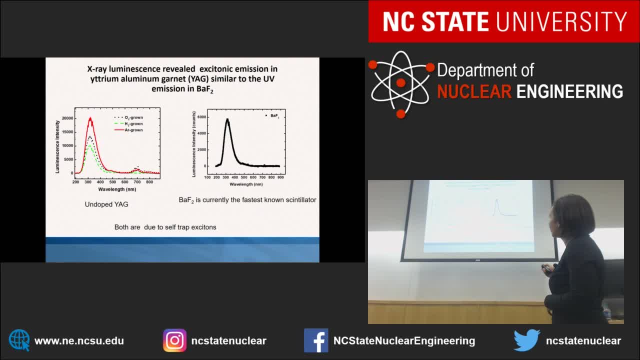 this detector because we call it Yttram aluminum garnet. Yttram aluminum garnet YAG is again an important material. There's a lot of effort to develop cerium YAG as an efficient centralator, because cerium YAG is a very, very very. 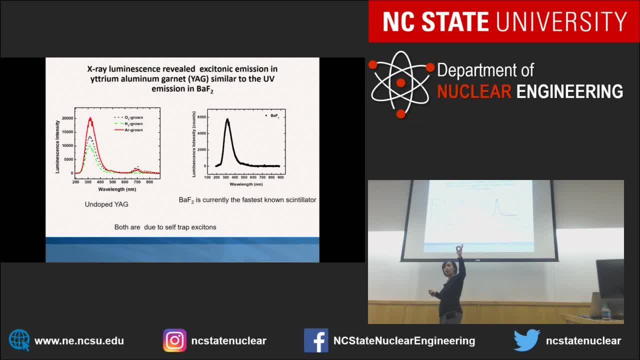 high efficient material. It's actually when you get the cerium YAG- this is the phosphor they put it on the. if you have UV sources, they put cerium YAG as the yellow phosphor when you get the green emission. So it's a very, very efficient. 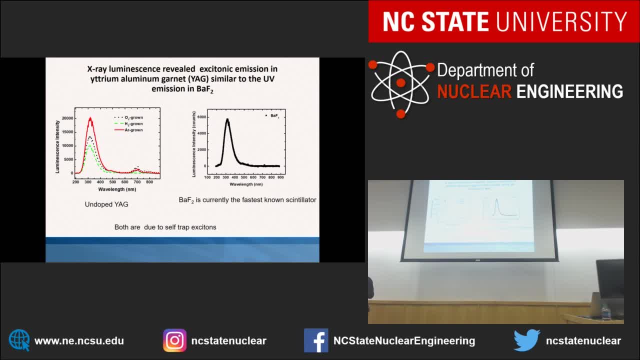 this. But it's hard to work as a centralator because of defect on it and defective traps, exciton, and you don't get good emission. So we've been working on this, but then we found that the end of the egg has really some interesting. 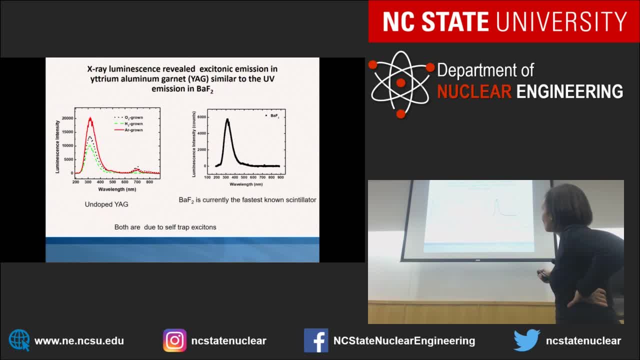 properties, So barium fluoride, for example. we were starting this by this spectrometer. we developed X-ray induced luminescence and here's the barium fluoride detector. So the emission you get here around 300 nanometer and the 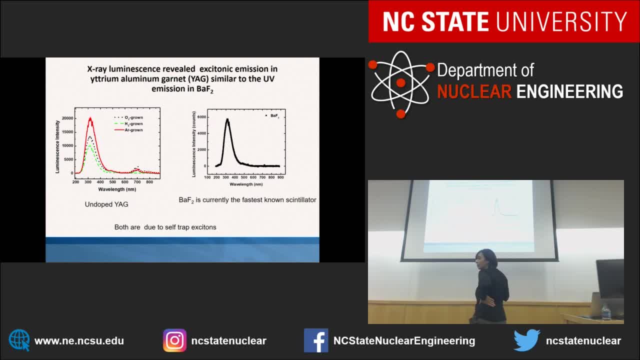 barium fluoride has one very fast emission which is people use as a fastest detector. so far Barium fluoride detector and the plastic centralator is the best, is really the faster detector. So if you want applications with high timing resolution you need this kind of detector. So people have been using the barium. 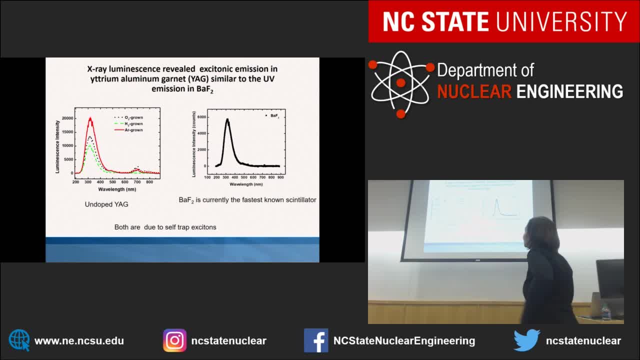 fluoride for this so far as the fastest known centralator. So we looked at the end of the egg and we find we have this emission similar to the barium fluoride. and you see, by different, by different treatment, we are actually able to. 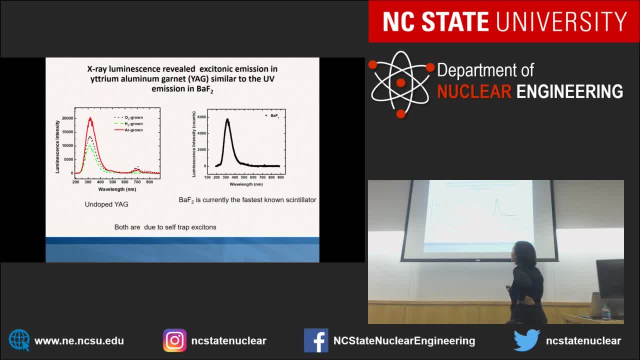 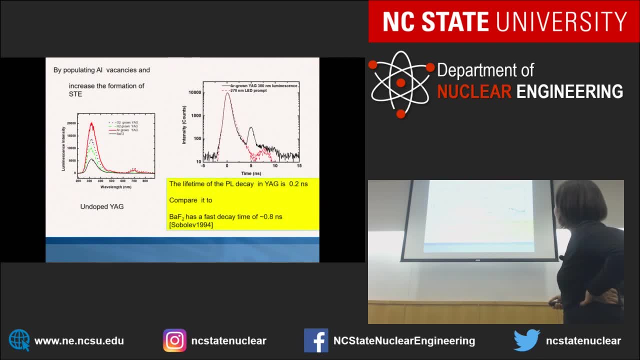 increase this emission from the material. When we treat the materials different- annealing- we're able to increase this and we also look to the lifetime of this emission. So we found that in the egg the lifetime is this: 0.2 nanosecond compared. 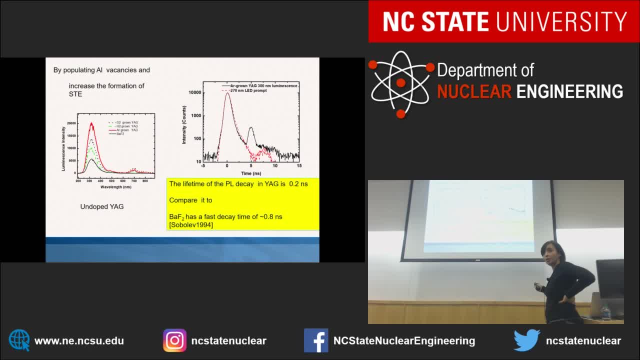 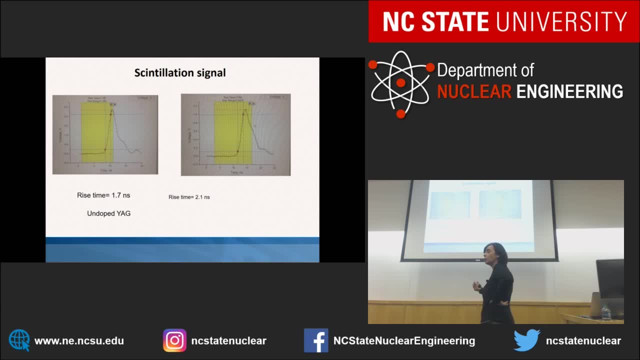 to the 0.8 nanosecond in barium fluoride detector. So if you look to this here's here then we detector. So very much we made. we constructed the egg, we connected to the hamamatsu photomultiplier tube and we connect also the same. 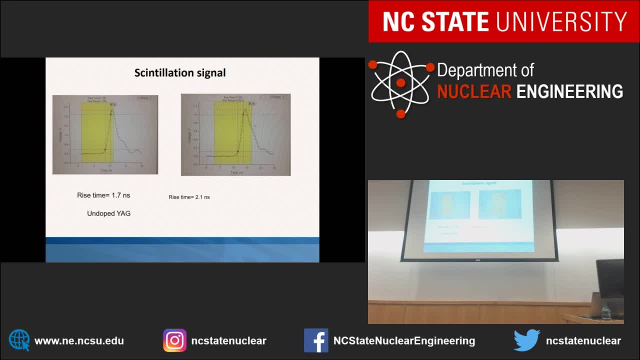 barium fluoride to the same hamamatsu bond tube and we did. we exposed them to gamma ray to see how it work as a scintillation detector And this is the outcome: found measure on the oscilloscope You can see. here is the rise time for the two. 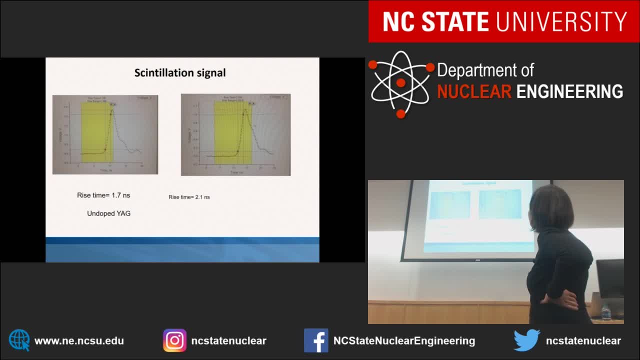 so for undoped the egg, we have 1.7 nanosecond. for the, for the barium fluoride, we have 2.1 nanosecond. So this is very much the same. I don't want to actually. 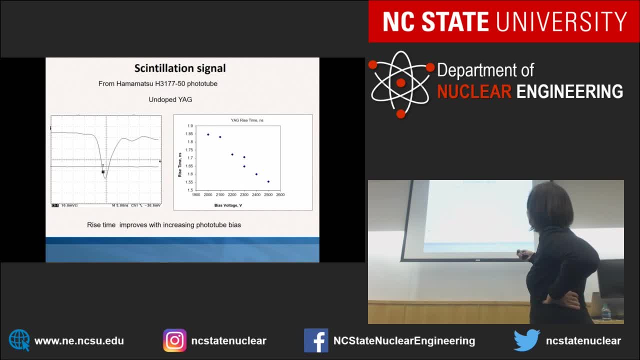 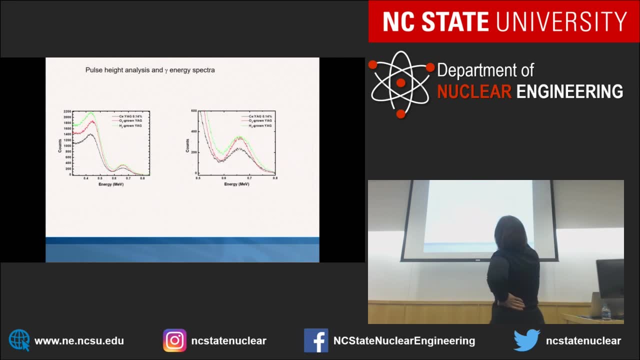 let me go skip here and show you the energy resolution. This is the. this is peak measure by the cerium egg and by by by undoped the egg. Let me show this is the one that's important for me to show you, because this is peak. 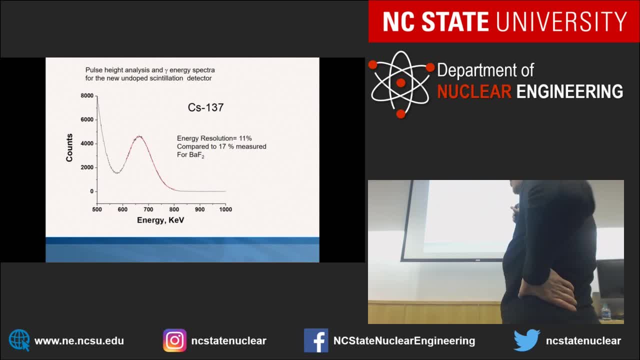 This is 662 kiloelectron-valve peak from cerium source and we measure this with our new detector, which is the undoped the egg, and we get very good energy resolution for this peak, which is 11%. 11% is very good energy resolution with a. 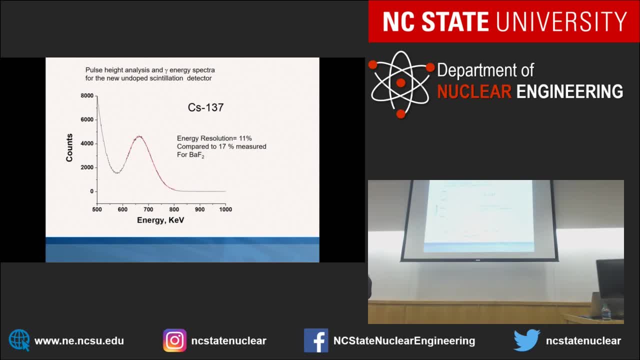 very fast detector compared to the barium fluoride. So barium fluoride- actually the energy using barium fluoride, is 11, 17%. But for this one we have a very good energy resolution: we show it's 11% and it's a much faster detector. So this is some. 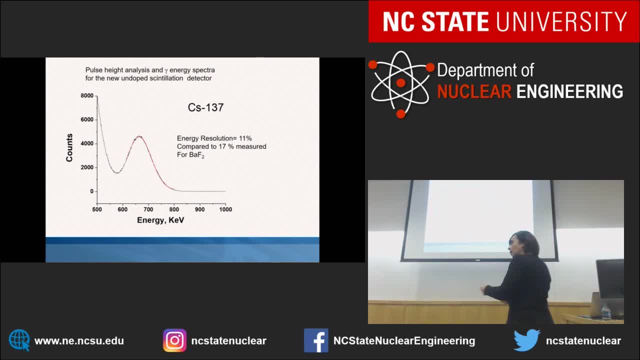 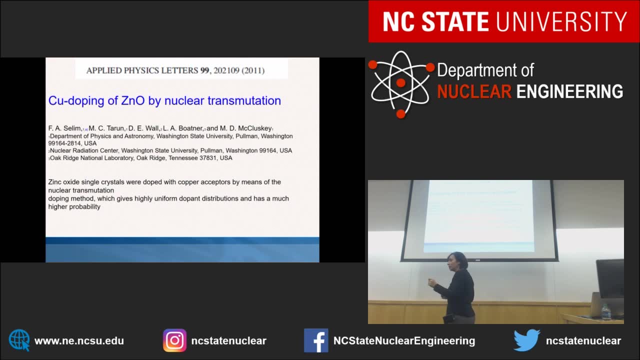 of the stuff we're working on to develop new centralization detector for this peak. We don't really use positron here. The last thing I want to mention, probably when I when I talk to you, Scott, about what interesting stuff we're using in nuclear reactors. 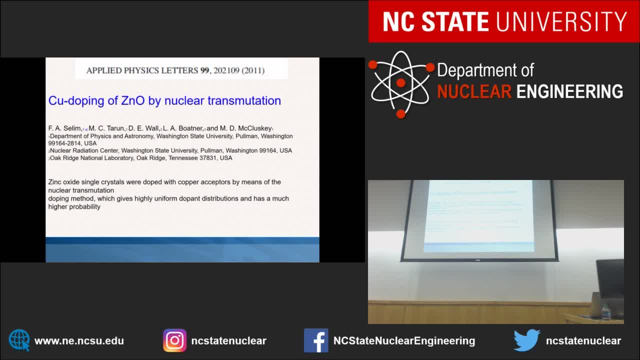 Some of the actual stuff we're doing. we use a nuclear reactor very much to dope semiconductor material. You know people have been using this in silicon to dope silicon. But we start to look to oxide and some of the stuff we did was dope zinc oxide. 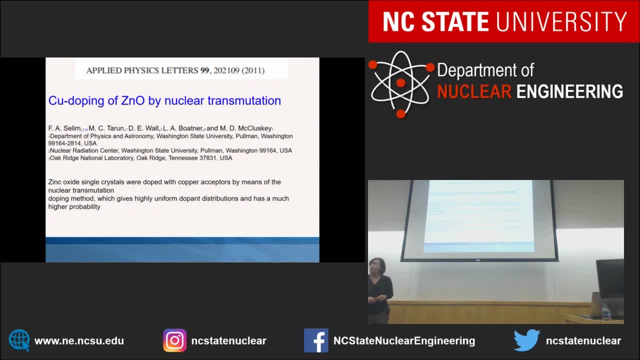 We want to dope it with copper and we just. it's about when you do it by the normal, normal way, it's always harder to get the copper to stay and the zinc is sublattice. So it's always go to the interstitial places, or? but if you have the zinc itself, you can. 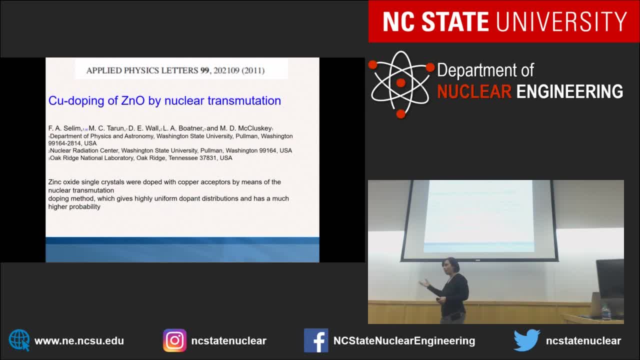 transmit the depth, the zinc, to copper, And this is when we know that you need, of course, a thermal neutron to do to do kind of this stuff, But you can really transmit some of the here, for example zinc, We're able to make. I didn't show this work because I didn't remember. 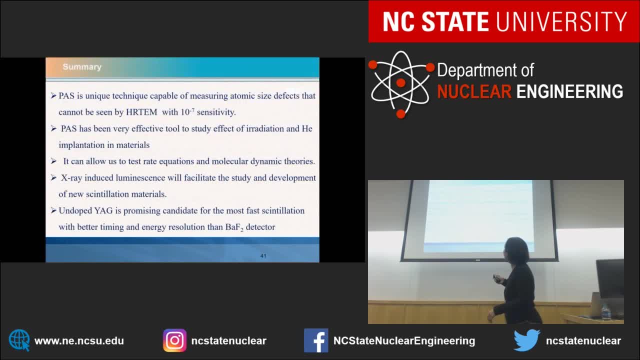 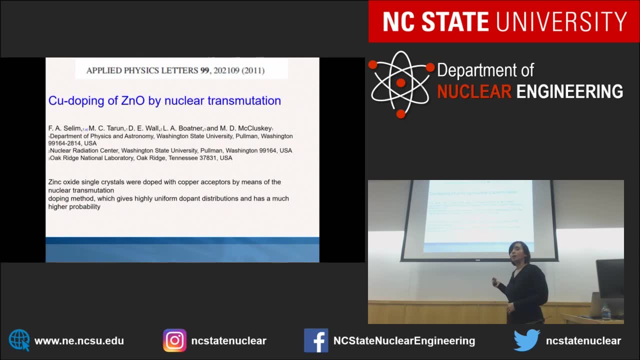 until I talked with you that this is some interesting area for for application of nuclear reactor and material science that really used to dope a lot of this interesting oxide. So anyway, this is we had. we all had a lot of questions. 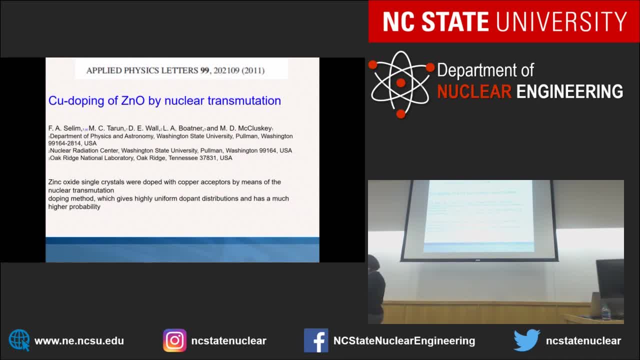 We saw very nice work actually and- and this is big area, by the way- We first we published the first paper in 2011,, but several people actually follow this and they started to do special on and dope zinc oxide with copper and this and the study. 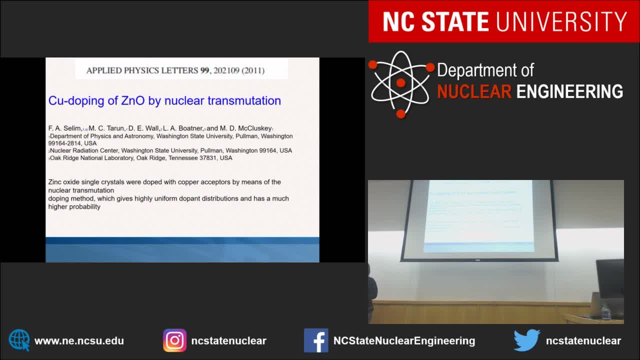 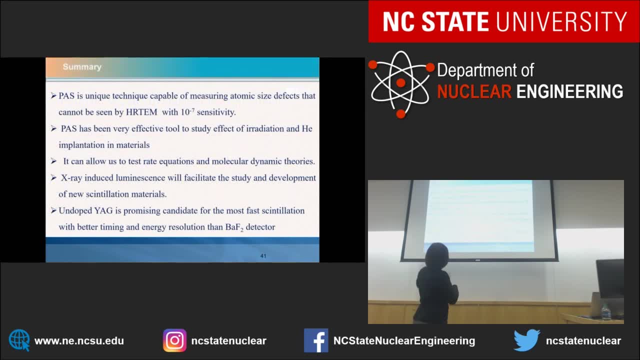 with with the stuff. So it's it's important this area in in term of semiconductor material and how we dope semiconductor material. So anyway, let me, I guess I'm done. So this is a summary. I guess I don't want to you. you can read it. 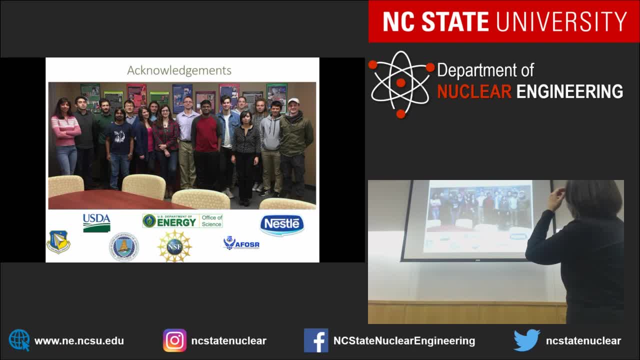 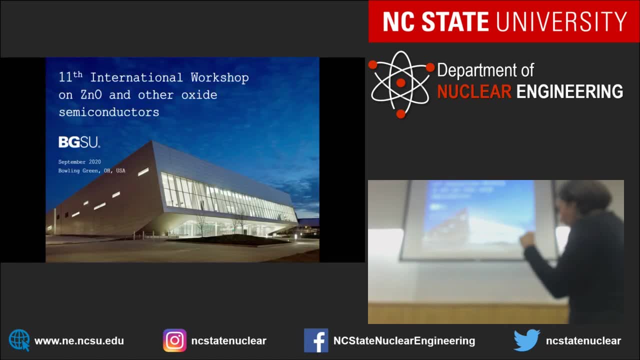 And I was just going to give give acknowledgement to for my student and our funding agency And sadly I want to tell you we are hosting actually the- I don't know if anybody's interested in oxide here. We're hosting the International Metering of Zinc Oxide in Bowling Green, 2020.. 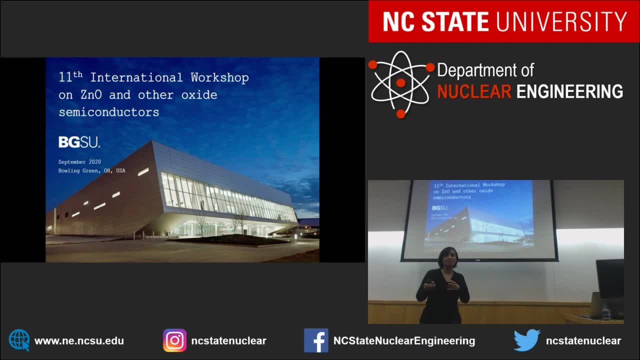 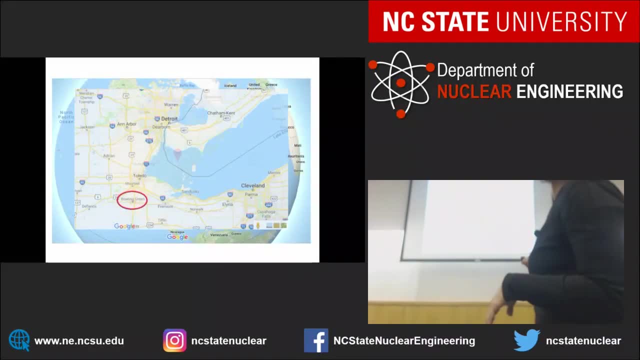 And it's also very zinc oxide or all oxide semiconductors. Probably the area is a little bit far from you, but just want to mention it And I can't tell you here where we're here. We're located here. 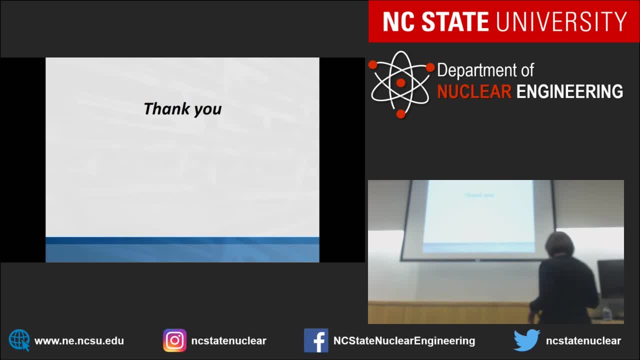 And thank you for your attention. Is there a quick question for Professor Simmons? We have a few from the professors, maybe from the students. Yes, So in in the first slide you mentioned working on zinc oxide. Do you grow this in your lab? 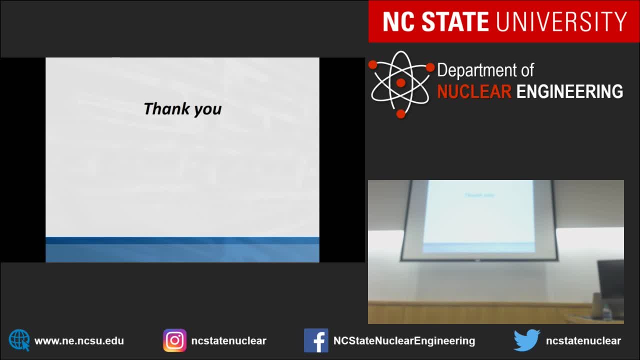 Yeah, I do metal, or you probably. it's a good question because how you know how hot gallium oxide area is? Yeah, we grow gallium oxides with metal organic chemical vapor deposition. This is really our main use. It's a very important for higher power transistor.